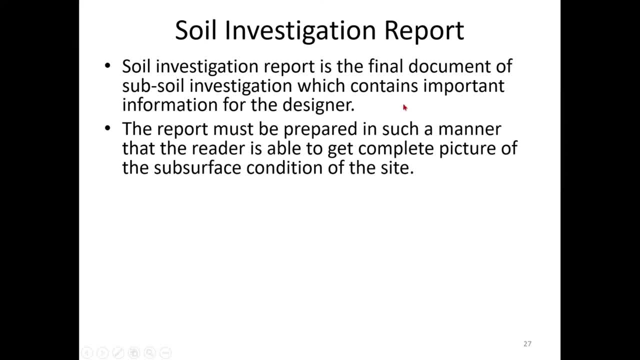 information for the designer. So, based on this site investigation report, the designer will design here. So they will decide what is the load bearing, they will identify what is the load bearing capacity of the soil, what is the type of soil, what is the depth of extent of that soil, what is your? 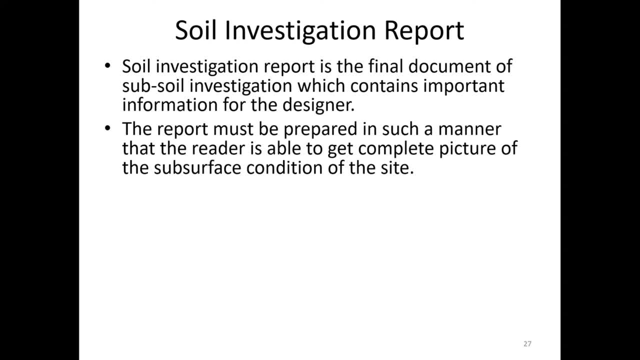 superstructure load. how wide your foundation should be to transfer that load safely? can the soil beneath carry that load safely? will the soil settle? if this happens? will the fluctuations in groundwater affect that soil? is dewatering required to be done at the site? So all these 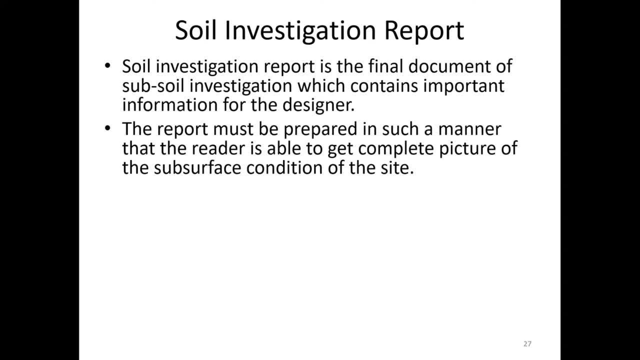 information should be, you know, provided by the geotechnical engineer, based on the soil investigation report. So you should. if you are looking at a site investigation report, you should have a clear idea about all the subsurface soil profile, occurrence extent, etc. Right, So a good. 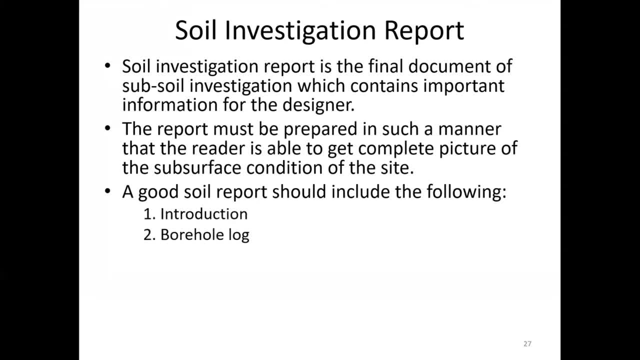 soil report should have the following: It should have an introduction about the site. It should have a borehole log. I will show you what is a borehole log. It should say what is the method of investigation. you have adopted A few investigation methods. we already saw yesterday right auger boring. 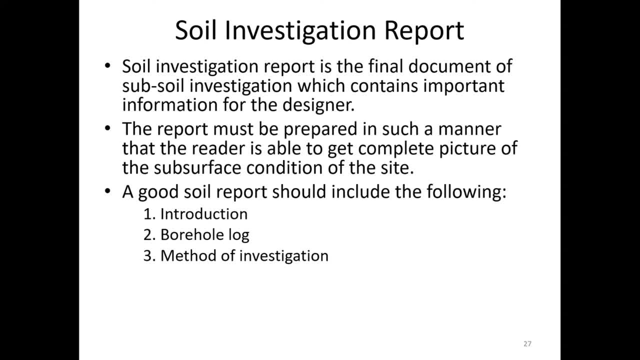 shell boring, rotary wash, percussion, etc. So what is the method of investigation adopted at the site? and once you have collected the soil samples, what are the test results for that sample? So then, analyze. you have to analyze those results and you have to give your recommendations right. So, based 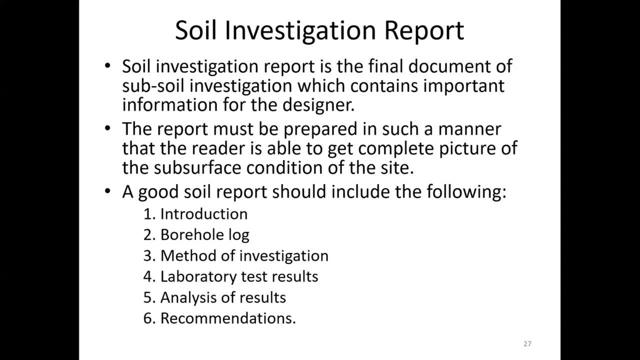 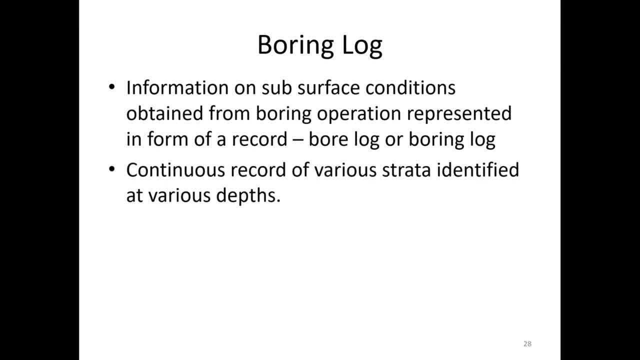 on this. a geotechnical engineer will design your foundation. okay, A borehole log or a boring log I have mentioned yesterday. you are continuously going to, you know, dig into the soil, or you are going to make a borehole in the soil and you will identify what is the type of soil under the ground, what is the extent of the soil in the ground and at what depth. you will identify your hard rock strata, etc. So all these data should be entered into a bore log. That should be made into the form of a bore log. 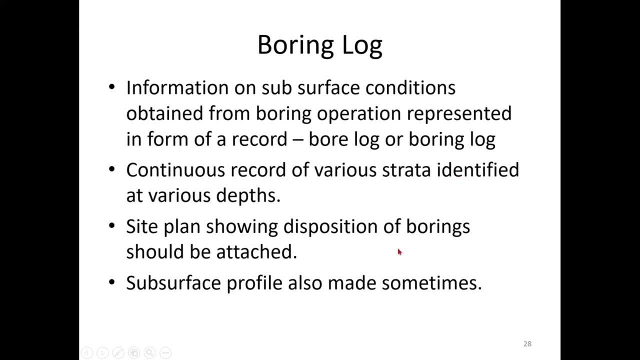 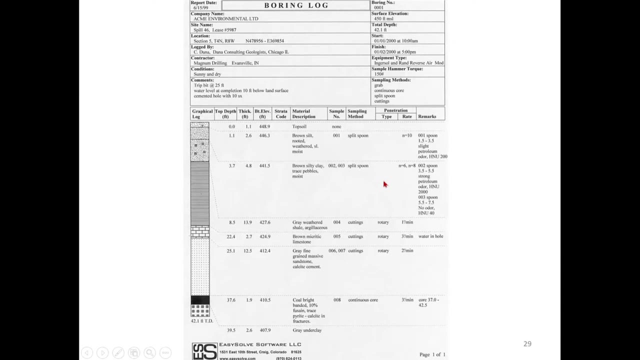 of a record. So that record is called a bore log or a boring log. So it is a continuous record of different strata identified at different depths right And also in a boring log you should also show the site plan showing the disposition of boring locations. So sometimes a subsurface profile is also made based on the bore log data. So this on your screen you can see a sample boring log. So you can see here the date is there, bore number is there. 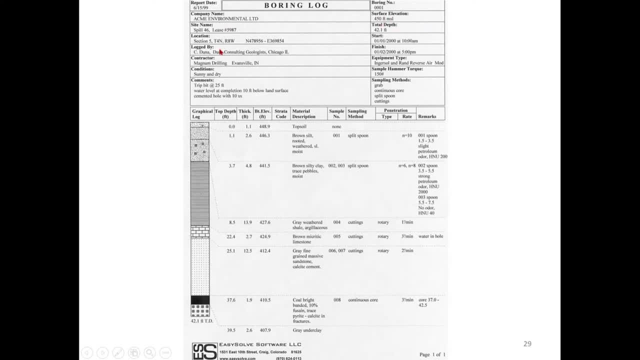 company name, surface, elevation, depth, site name, location of the site, who logged it, starting time, finishing time, who is the contractor, equipment type, what is the equipment they have used- sample hammer, torque condition, site conditions, comments about the site, sampling methods- all these data will be there. Then, the most important part, this is the bore log. So this is your graphical bore log. Okay, so here you can see. So this is the on top. this is your ground surface. So top depth. 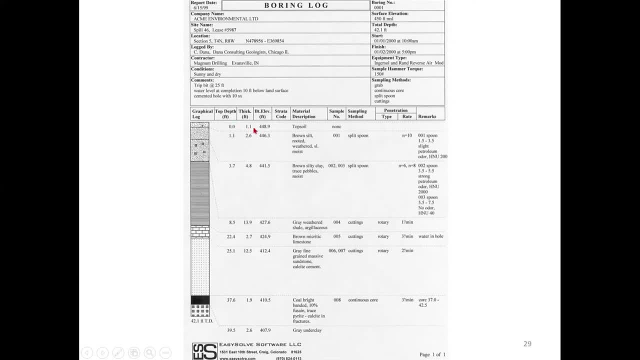 0.0, right. So from 0.0 to 1.1 meter. so this much depth is 1.1 meter. So till 1.1 meter. you had top soil, Okay. So the top soil sample was not collected. we don't need it. 1.1 feet, only very small thickness and top soil. we are not collecting the sample because we are not going to rest our foundation on the top soil. All right, So from 1.1 meters to 2.6 meters. what soil do we have here? This one. 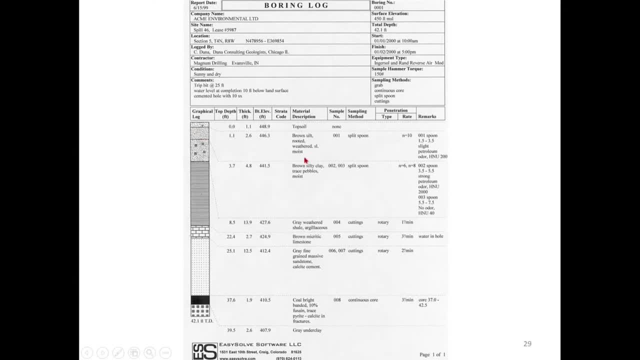 We have brown silt, rooted, weathered and moist, Right. So this soil sample has been collected and it has been assigned sample number 001.. And how did they sample the soil? They use the split spoon sampler. I'll show you a split spoon sampler and how sampling is done. All right, Then you have penetration type and rate. Okay, So here it is mentioned, n is equal to 10.. So n is the SPT number. I'll show you what is an SPT. 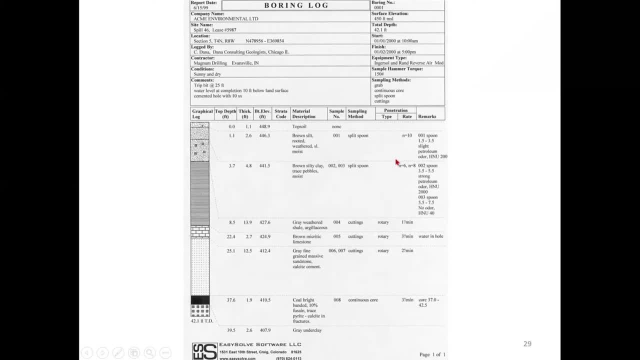 SPT standard penetration test. So for that standard penetration test, how many number of blows was required for penetrating to a particular depth that is represented by the n number? Okay, So penetration rate: it was n is equal to 10.. Okay, And using a split spoon sampler, the sample was collected from this particular depth. Okay, So any other remarks? So they haven't mentioned the remarks. 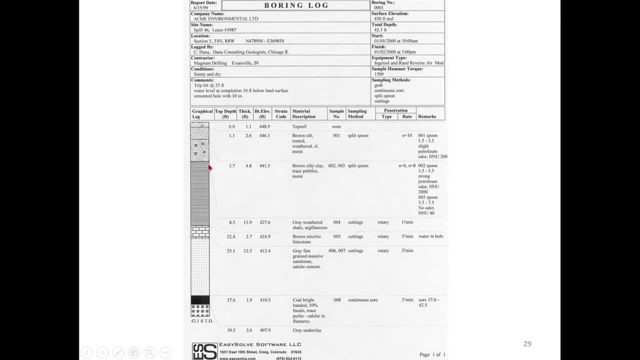 So from 3.7 meters to 4.8 meters you have the next soil. They have represented it with the different symbol. Right You have another soil from 3.7 to 4.8.. So that also material description. This is what you observe. Okay, This is based on the observation at the site. So it is a brown, silty, clay, trace pebbles and it is moist. Okay, Two samples were collected, Sample number two and three, Again, split spoon. sample method N: numbers are noted down. Similarly, next strata: you can see it is a pretty deep strata. 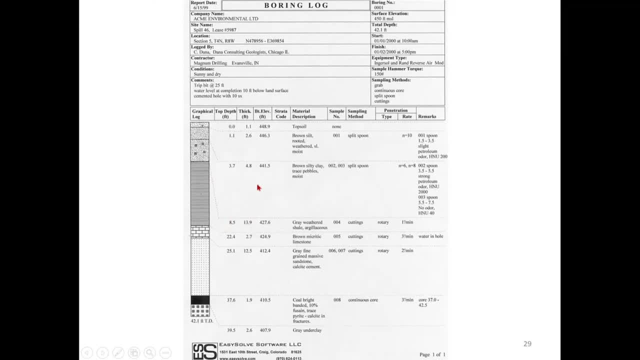 It is 8.5 meters until 8.5 meters and the thickness is 13.9 meters- sorry feet. and it is grey, weathered, shale or gelaceous material. So samples were collected. Sampling method: it is cutting. Okay, It is not split spoon sampler. I will show. 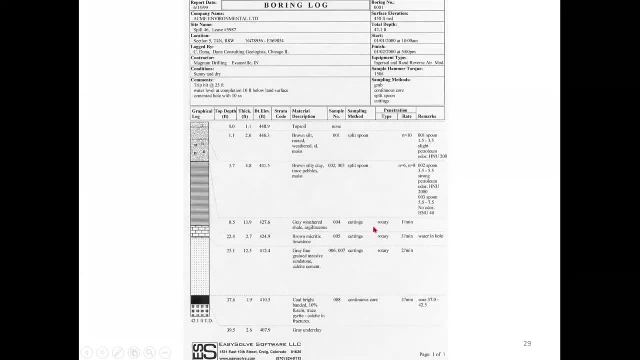 you cutting? Okay, And penetration type? can you see It is rotary drilling, Right, Rotary drilling we saw yesterday, Correct. And another remarks: water was there in the hole. So like this you will make a complete list of the subsoil, uh strata and its depth of occurrence, its extent occurrence and its 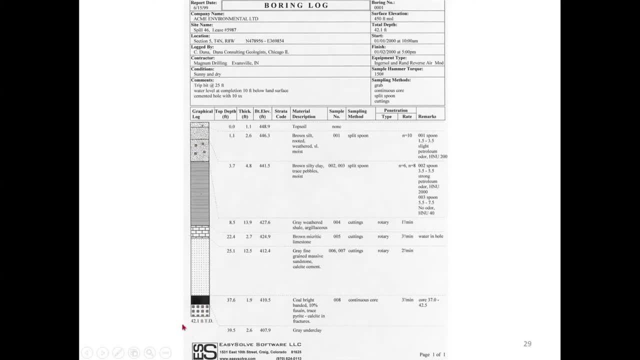 extent will be marked graphically like this: okay, and here, finally, at 39.5 meters, and until 2.6 meters, they have continued the excavation. so it was found that at that level you have gray under clay. all right, so maybe, uh, this here the total thickness and depth until which they 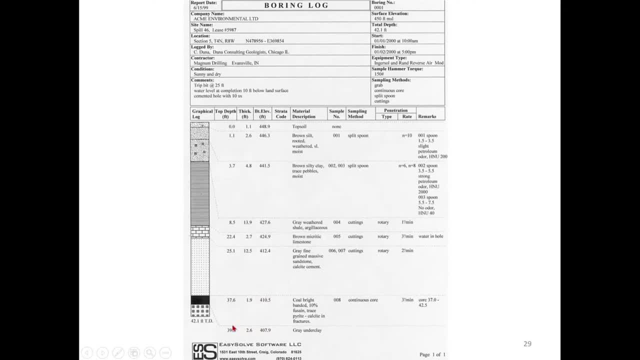 have conducted. this is about about 40 meters, right? maybe this depth was enough for that particular foundation, for maybe a single storage structure or a two or three storage structure. but if it is a very- you know very- heavy structure, you might have to go for a boring until you reach your. 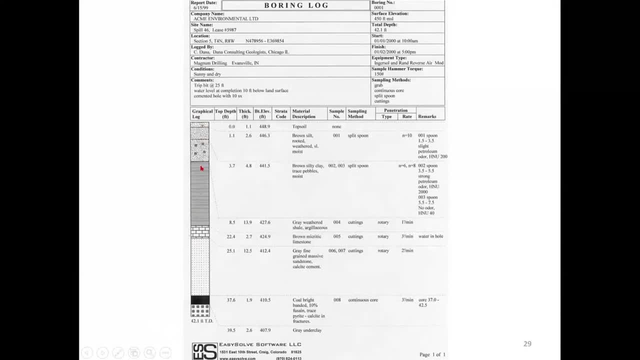 hard rock strata. so, till the hard rock strata, you will continuously make this log of what all are these different types of soil available at the site. okay, so this is a different detail boring log. okay, this is very important. this carries about 20 marks in your semester i. 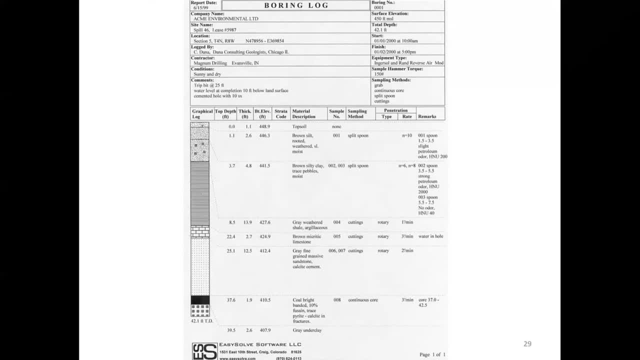 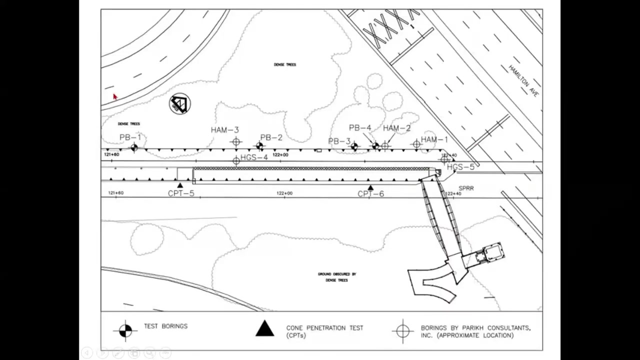 think i have mentioned in your initial evaluation pattern that you will have to develop a geotechnical report and recommendation, so this is one very important parameter for that. okay, we will discuss that later. okay, so keep this in mind. so this is a sample boring log and this one shows the. 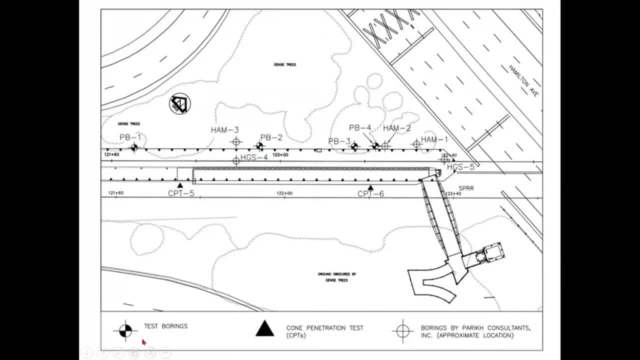 borehole locations, as you can see here. these symbols test borings. these are all the. this is the site plan. okay, this is the site plan. so in the site plan you will mark the boring locations, as you can see here. you will mark all the boring locations, then cone penetration test. that is. 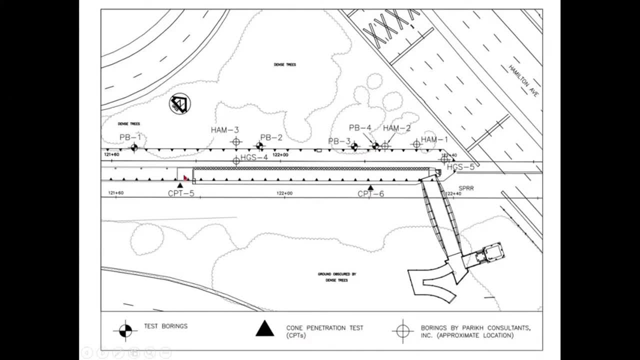 another type of penetration test. so locations where cone penetration test was carried out is also marked, okay. and another one: these are also borings- borings done by uh parikh consultant. someone else have done those boring so that locations are also marked, okay, this is a map showing the location of boreholes in the site. all right, you can see the north arrow. 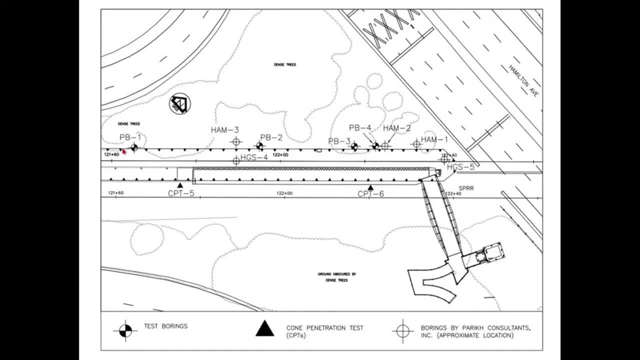 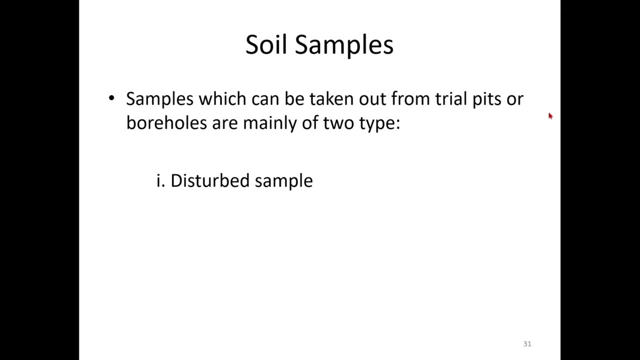 and all okay. so this is the site disposition and where all the moorings has been done. so this is also a important uh input in the geotechnical report or site investigation report. so different types of soil samples that are collected from a site. we had discussed it here and there earlier. 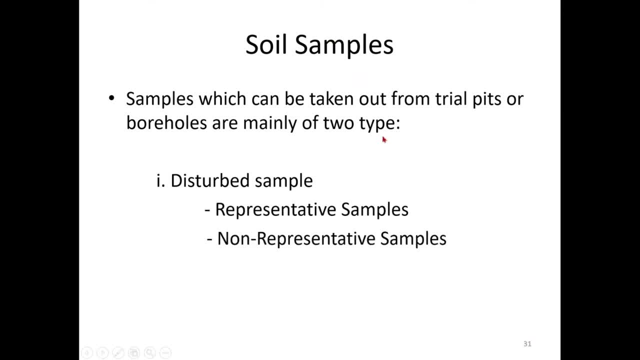 so you all know what are the two types of samples that can be collected from the site. so one is a disturbed sample and the other one is an undisturbed sample, right? so in disturbed samples we have two samples: one is a representative sample and another one is a non-representative. 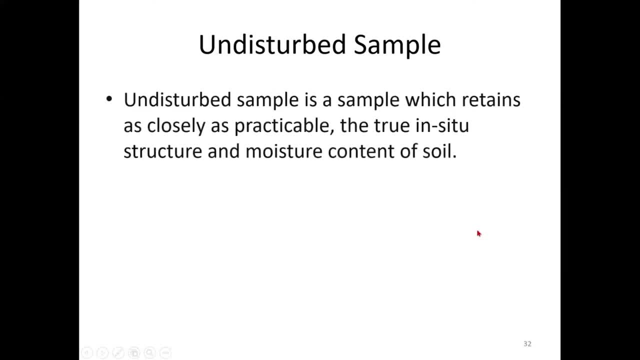 sample. so we all know what these are undisturbed samples. what are undisturbed samples? so a sample which retains as closely as possible the true in-situ characteristics of the soil and the moisture content. right, the soil sample which is as closely representative of the 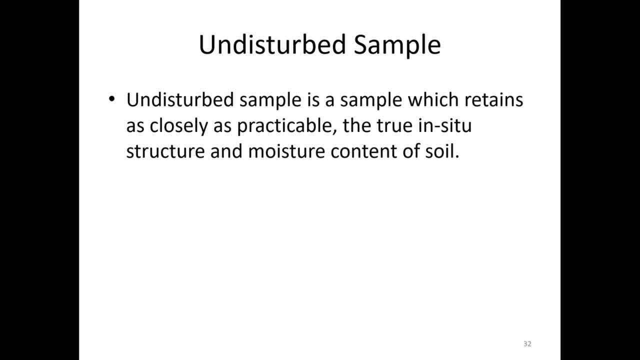 soil condition is the site sample soil condition that is called a undisturbed sample. right, this undisturbed sample is going to represent your site condition. uh, most uh practically, or most uh closely, as closely as possible in the lab. okay, so that's a undisturbed sample. 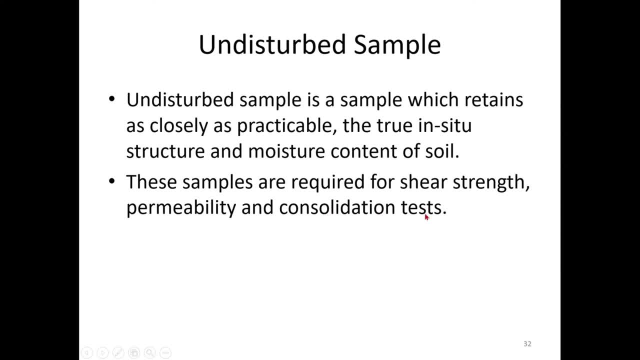 so this: samples are required for shear strength, permeability and consolidation tests. right, these three parameters. you can see these are the engineering properties of the soil, so they require undisturbed samples, right? so if you want to identify the shear strength, permeability and consolidation properties of soil at a site, you have to collect undisturbed samples. all right. 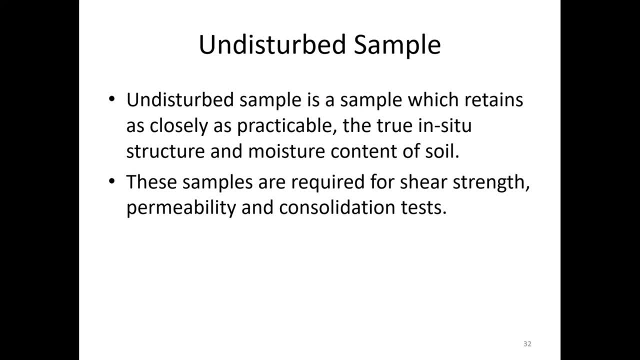 so what can we use disturbed samples for? you can't use disturbed samples for a permeability or consolidation test- right, because it will already be, or shear strength test, because it already will be very much disturbed. the soil structure will be altered, moisture content will be altered, it might have mixed up with different strata or different types of soils, etc. isn't it? 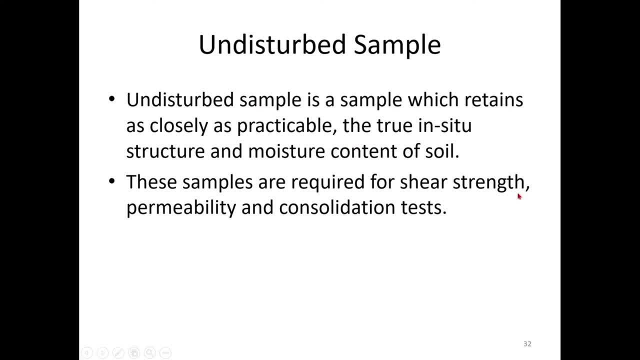 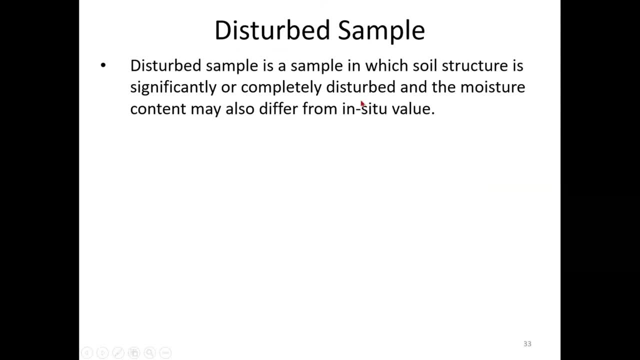 so what can you use a disturbed sample for? let's see so disturbed sample. there are two types of disturbed sample. so in the disturbed sample it's a type of sample in which the soil structure is significantly or completely disturbed and the moisture content also may differ from its in-situ. 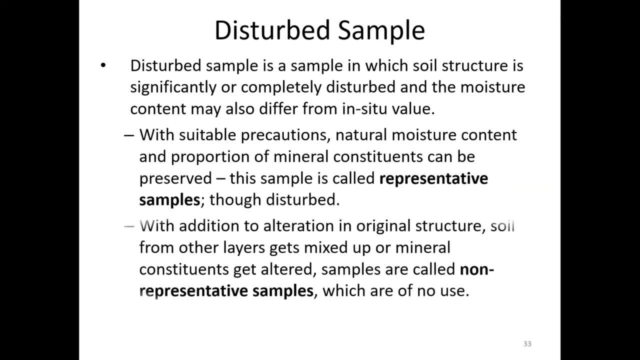 value. so there are two types of disturbed samples. one is a representative sample and a non-representative sample. so if you can, if it is possible with some suitable precautions, you can retrieve a disturbed sample from the site. but still you can make sure that the natural moisture content and the 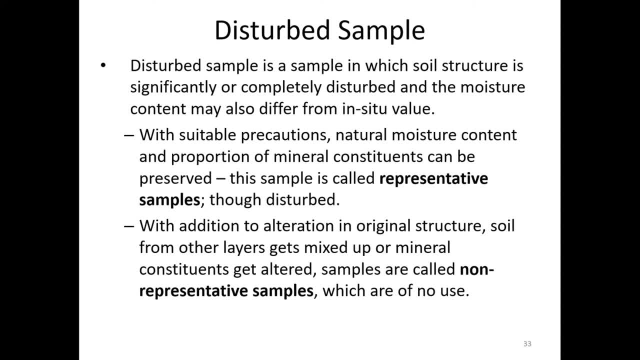 proportion of mineral constituents are kind of retained or preserved. so those types of samples are called representative samples. you will make sure that it doesn't mix up with different layers of soil or it doesn't, you know, mix up with the ground water etc. so you will try to retain the 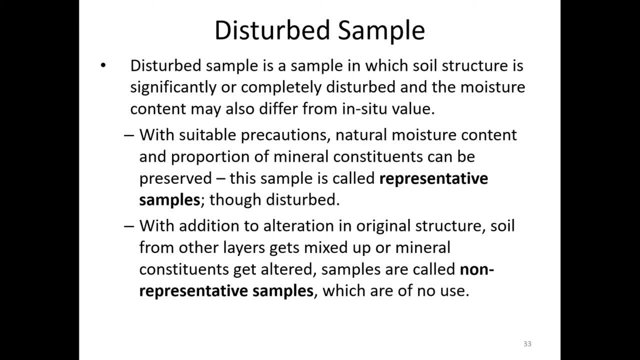 natural moisture content and mineral constituent proportion as closely as possible. so, but still the soil structure or arrangement of the soil will be disturbed and its- you know- soil structure or arrangement will be significantly or completely disturbed, but still you can identify its natural moisture content and mineral constituents from that sample. so those samples are called. 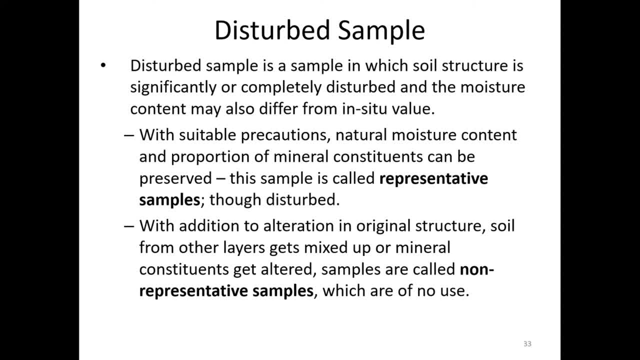 representative samples. even though they are disturbed, it's representative of a particular strata, right, but some soil, when you're collecting it, it will be. you know your all. your complete structure of the soil will be altered. it might get mixed up with soil from different layers. so the 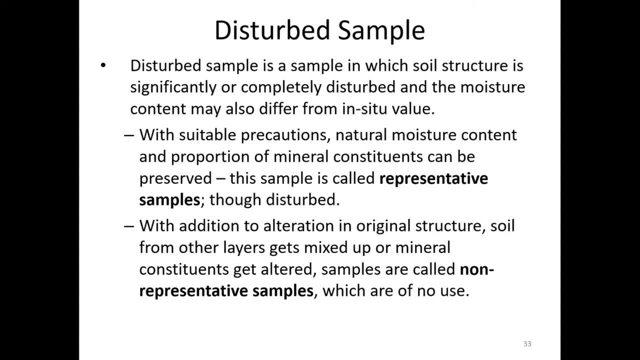 the mineral constituents are also altered, So such samples are called non-representative samples, which are of no use, right? So we have disturbed samples and undisturbed samples, and we have representative and non-representative samples in disturbed samples. Hope this is. 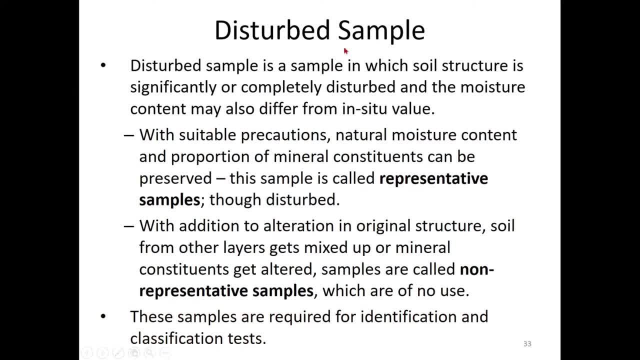 clear. So these disturbed samples are required for identification and classification tests. What are those tests? Passive test, particle size, distribution curve. then what other tests do you need? Liquid limit and plasticity intake, So for Atterberg limit test, soil identification. 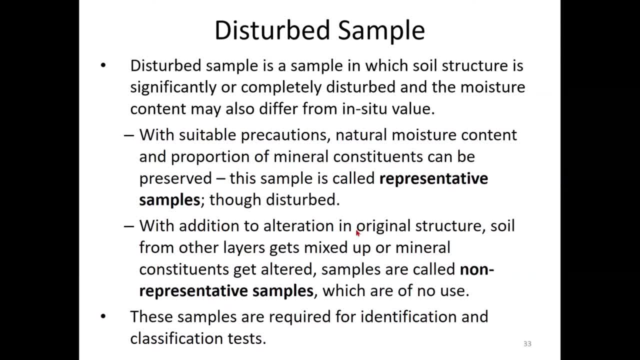 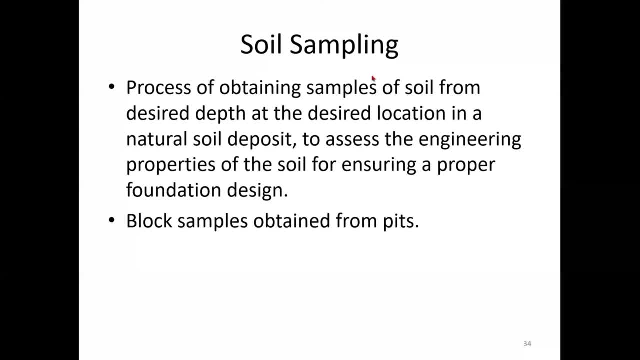 etc. we can use disturbed samples, all right. So next topic is soil sampling, how we are obtaining samples from the site. So soil sample is nothing but the process of obtaining samples from the site at desired depth and desired location, which is used for assessing. 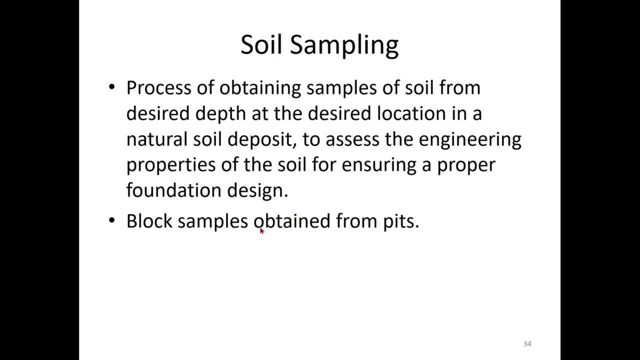 the engineering properties. So we have different types of samples. We have block samples, we have tube samples. all right, So block samples are obtained from the pits and tube samples are obtained from boreholes. So the devices used for obtaining 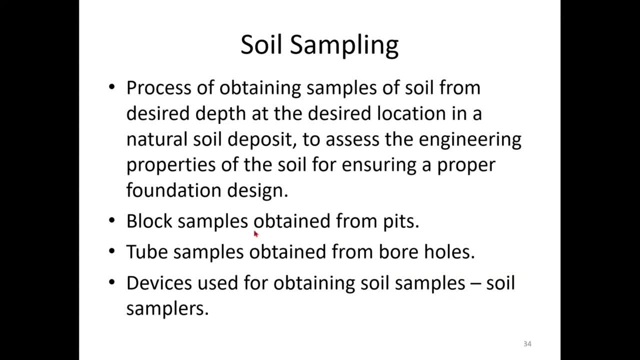 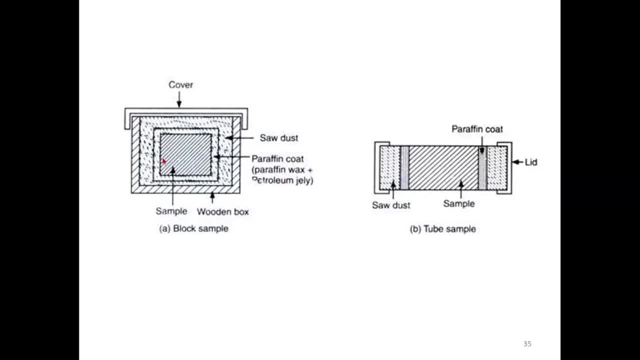 the samples are called soil samplers. okay, So I will show you a block sample. Here you can see a block sample which can be obtained from a pit. So block samples like this you can see here this hatched portion is my sample. So what I will have, I will have a wooden. 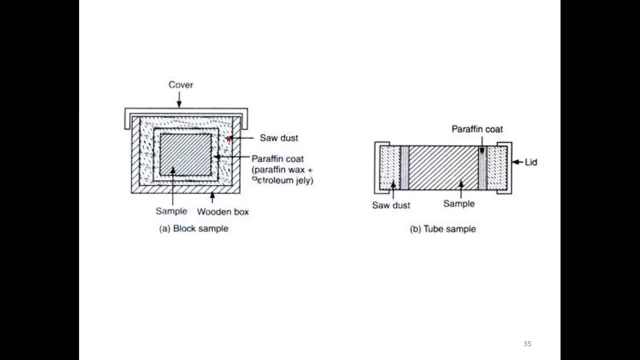 box like this. So inside the wooden box I will fill some sawdust, Okay, And I will collect a sample from the site. Then I will coat it with paraffin wax so that the natural moisture content is not disturbed. Okay, I will coat the whole sample. 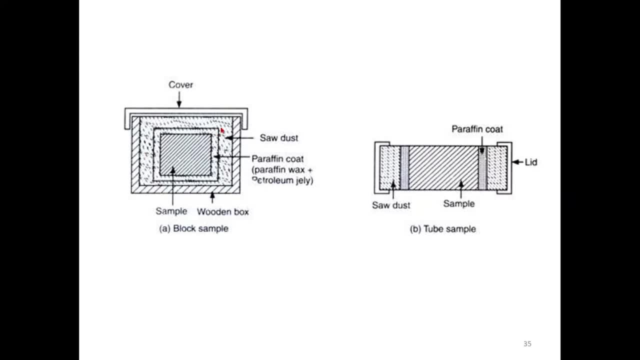 with paraffin wax, and then I will place it carefully within a wooden box which is filled with sawdust, so that the moisture content is also preserved and the sample does not shake much. all right, Its constituents or particle arrangement is not disturbed much. 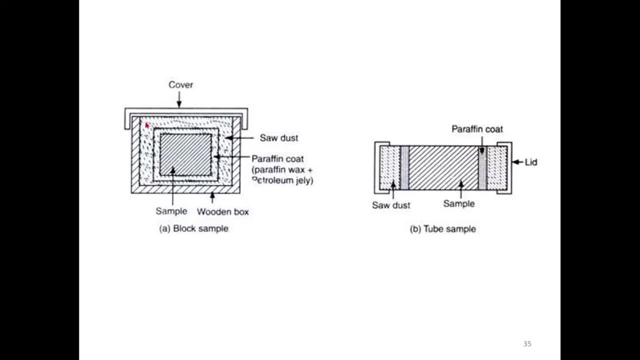 So this is a block sample, Then I will close it, I will fill it with sawdust, Then I will close it carefully, Then I will write the sample number, location details, everything on the box. I will send this to the lab So once it reaches the lab they will retrieve the sample. do different. 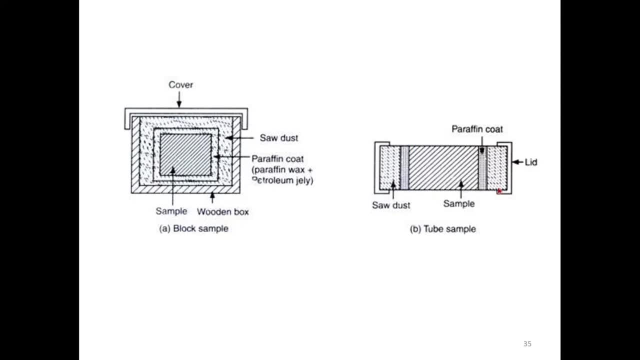 tests on it. all right. Similarly, you will also have a tube sample like this, okay, a small cylindrical tube. So inside that again you will collect the sample, Then you will coat it with paraffin wax on both sides, Then you will fill it with sawdust, So you will. 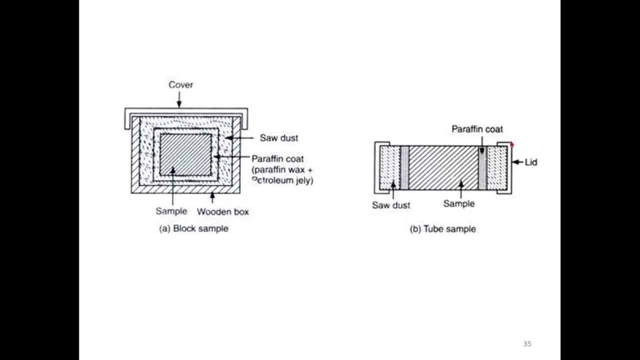 fill it with paraffin wax on both sides. Then again you will fill sawdust on both the sides. Then you will put it inside a container. You will have the lid. Okay, So there are two types of samples: block samples and tube samples. Block samples are obtained from pitch and 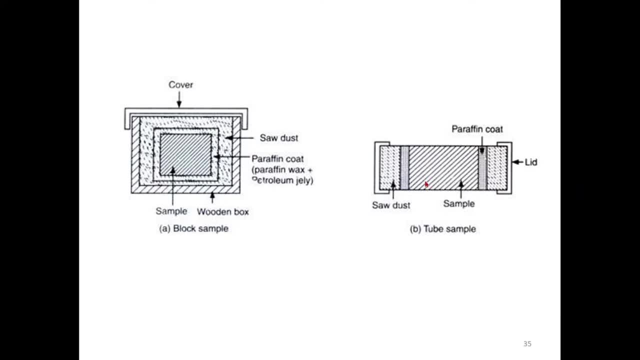 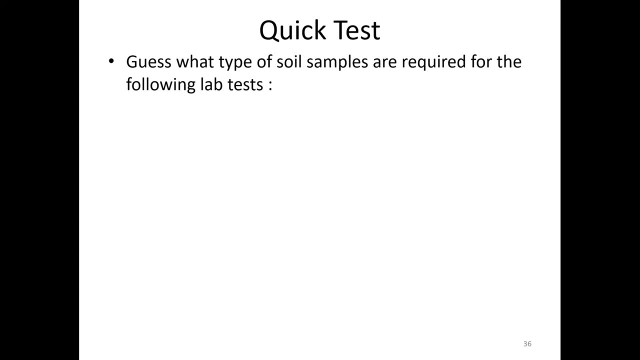 block samples are generally obtained from bore holes. Okay, So we will have a very quick test. So you have to guess what types of soil samples are required for the following lab tests. Okay, So soil samples are disturbed and undisturbed, representative and non-representative. 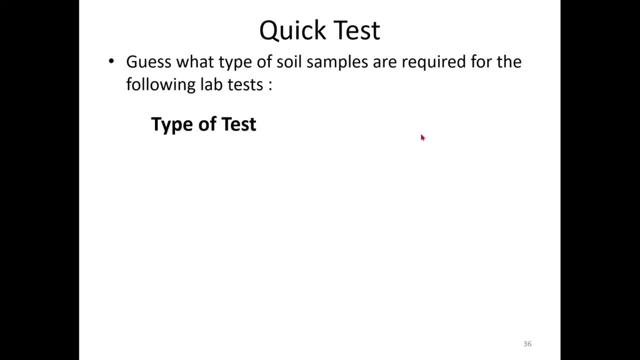 right. So soil samples are disturbed and undisturbed. representative and non-representative, right. So you have to carefully add them. So you have to tell me which one is needed for which particular test. okay, So different types of tests. let's see natural water content. 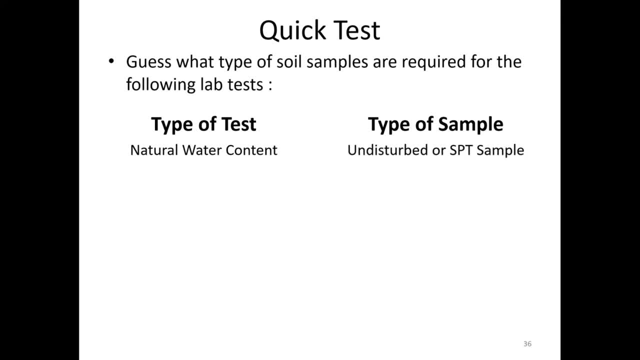 What type of sample do you need? Undisturbed or spt sample? Density of the soil: Undisturbed- Undisturbed. Specific gravity: Representative or undisturbed. Subjective, Deceptive, Gravitational or non- هنا Superb An un Monday Right. 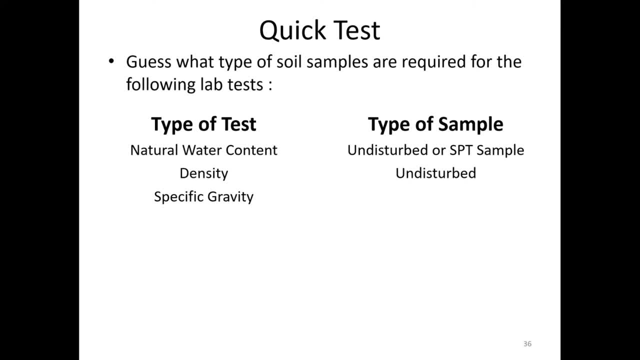 And we are going to do the values Next year. we have test Huang bater and what else. This is still getting ready. So, Coach pegs, Okay, Okay. Then we have a test for strat speaker. Good, later. trace sample: I have a simple scale sample: 10 m Вj. 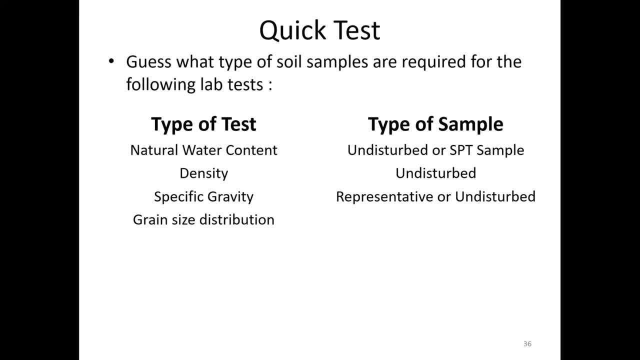 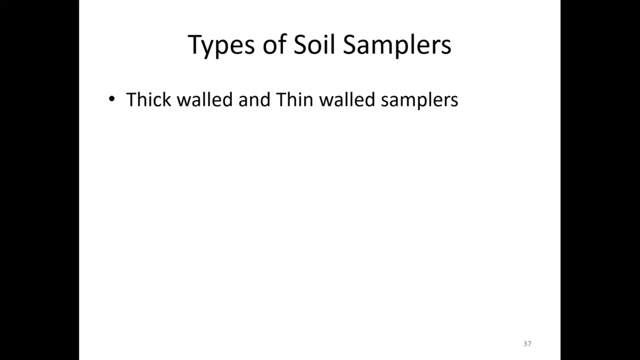 grain size distribution: undisturbed or representative. Atterberg limits: representative or undisturbed. coefficient of permeability: undisturbed only, then. consolidation: undisturbed only then. shear strength: undisturbed only. So there are different types of soil samplers. So we are talking about thick walled and thin walled samplers. 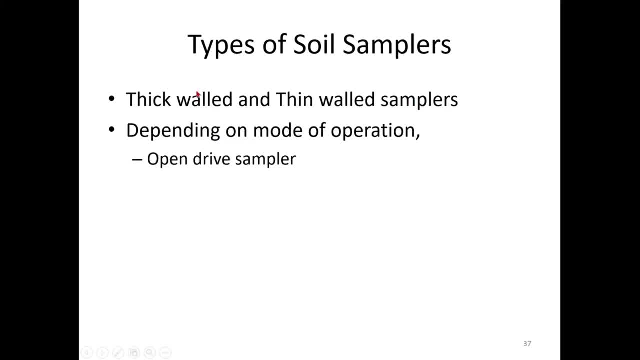 So, depending upon, we have two types of tube samplers. One is a thick walled sampler and another one is a thin walled sampler. And depending upon the mode of operation, we have three types: One is an open drive sampler, stationary piston sampler and a rotary sampler. 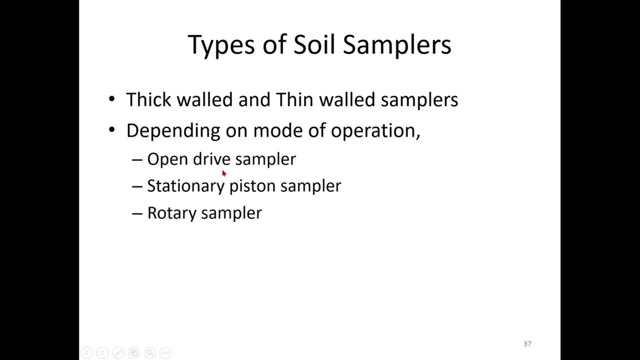 So open drive sampler. it is a split sampler. So this is a split spoon sampler which can be driven into the soil. Another one is a stationary piston sampler which will be slowly driven continuously into the soil without impact. Then the next one is a rotary sampler which will be rotated and cut into the soil. 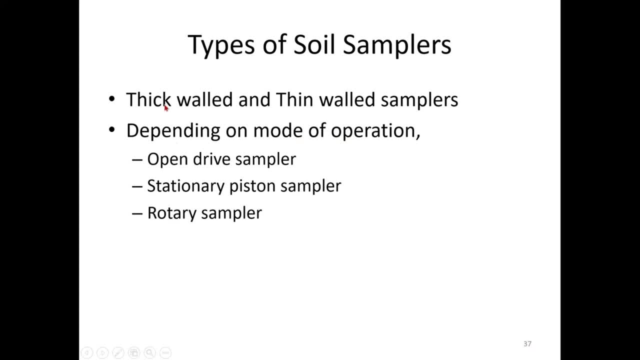 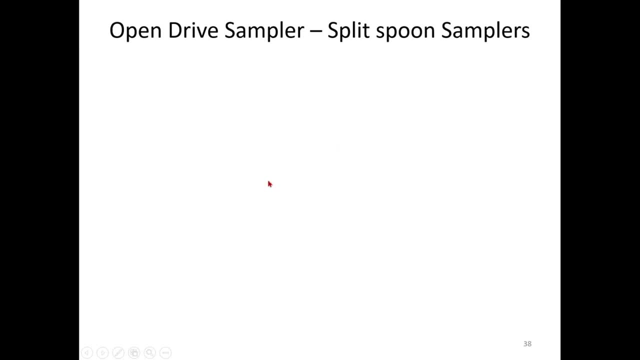 Basic three modes of operation. So you have two types of samplers. One is a thick walled and a thin walled sampler. So first let us see the open drive sampler or the split spoon sampler. I will show you a photo first so you can see. 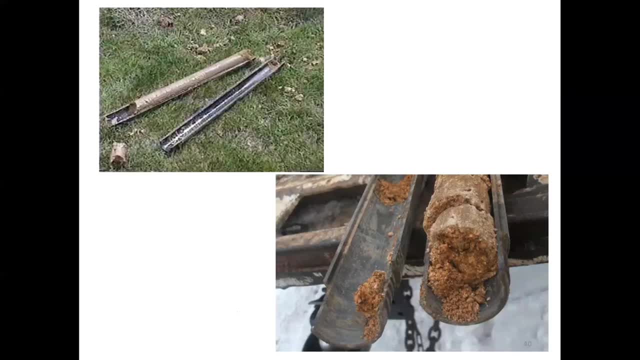 This is a split spoon sampler. I showed you this figure yesterday already. So this is a split spoon sampler. At one edge you have a sharp edge or a cutting edge, So this is closed. This looks like a pipe. This is driven directly into the soil and it is retrieved so that you will find a sample inside like this: 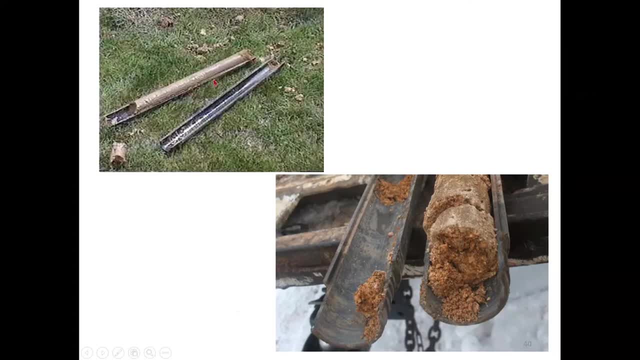 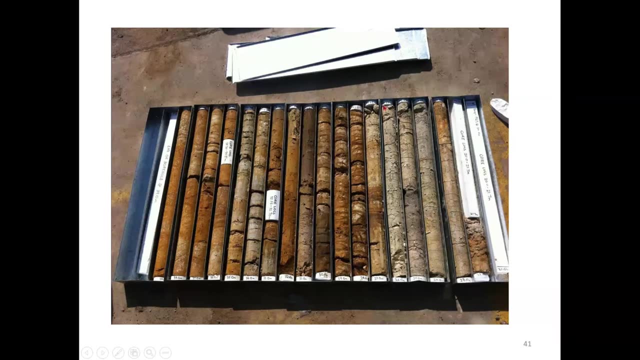 So this sample, you will close this again. You will either close this or put this in a wooden box like this, as you can see here. You can see this. then you pack this very carefully and you will send it off to the lab for further tests. 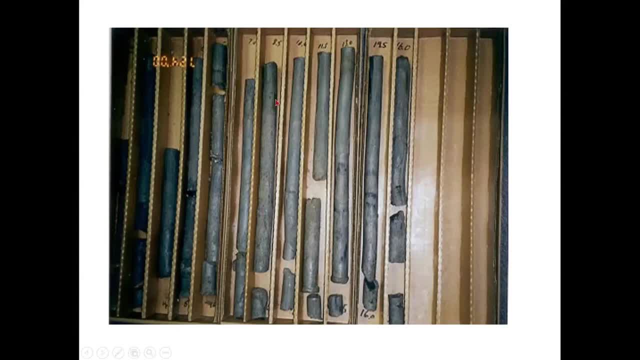 You can see here. you can see this: different samples collected from different depths Depths are marked here. Can you see this: at 7.5 meters, 8.5 meters, 10 meters, 11.5,, 13,, 19.5,, 16 meters. 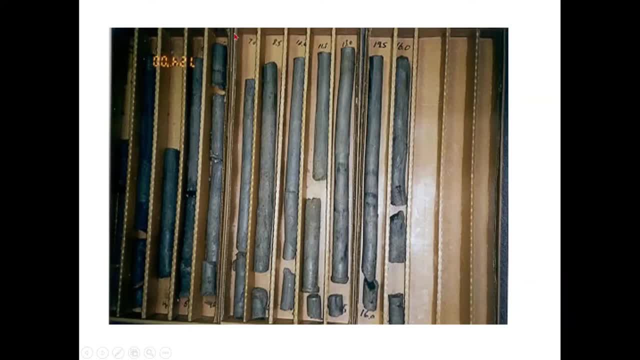 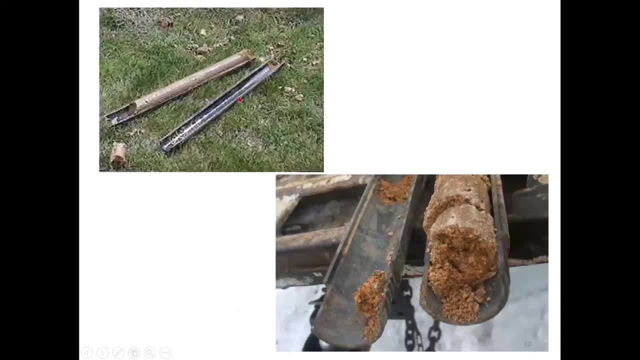 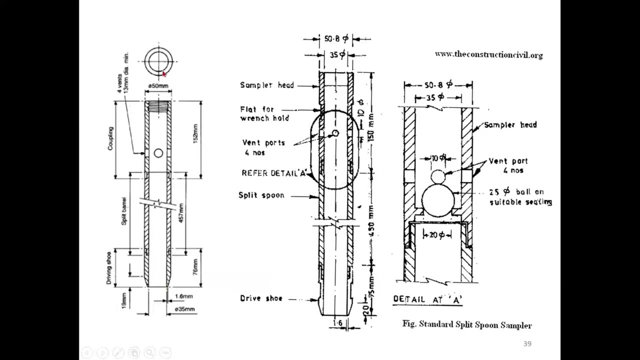 These are the samples collected at different depths, as you can see here. All right, So these samples or this sampler is called an open drive sampler Sampler or a split spoon sampler. Okay, It's very important. So this is a split spoon sampler. the closed section of a split spoon sampler. 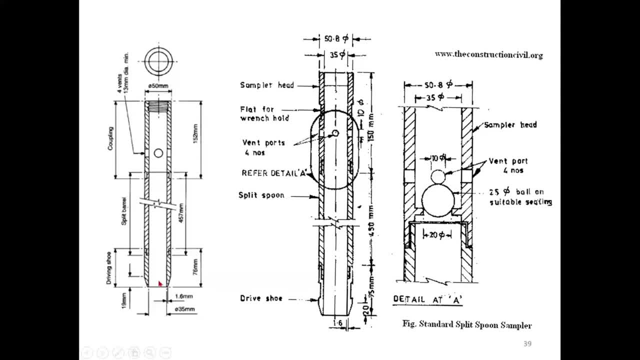 So you can see the different parts here. So here you have a cutting edge. You can see a sharp edge. All right, This is the cutting edge, All right. So then we have the cylindrical shaft or the sheath. Here you can see the threads. 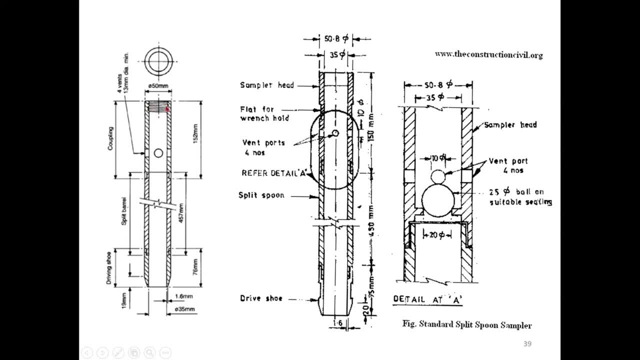 So these threads, it will be connected to the bottom of the you know drill. Okay, You will have a drill road. Do you remember the figures of wash boring, rotary drilling, etc. So, at the bottom of the drill road you will remove the churn bit or the cutting edge and you will connect this. 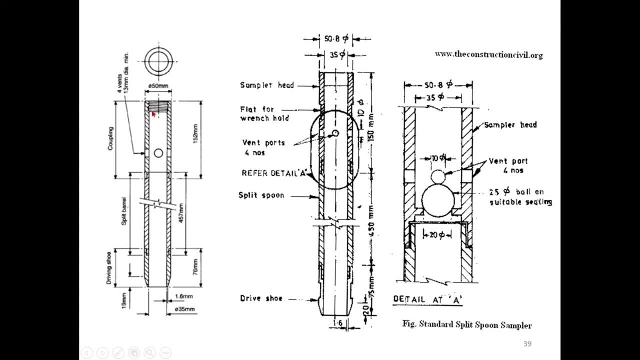 Okay, At the bottom of the drill road you will screw this on instead of the churn bit or the cutting edge, So you will fix this. Then you will drive this into the soil so that the soil enters this, And here you can see there are vents. 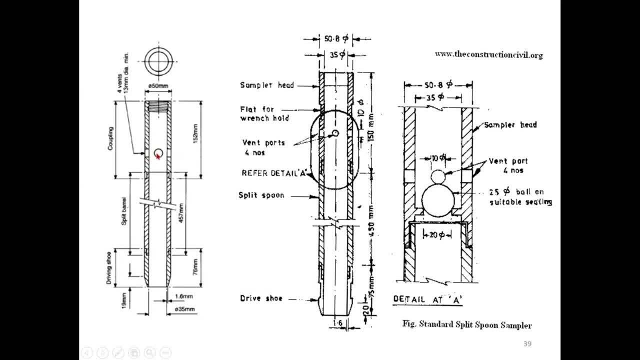 There are four vents on four sides. Okay, There are vents here for removal of air and excess water. Okay So this, you will drive it into the soil and the sample will be collected inside. Okay So it is a seamless, open end steel tube. 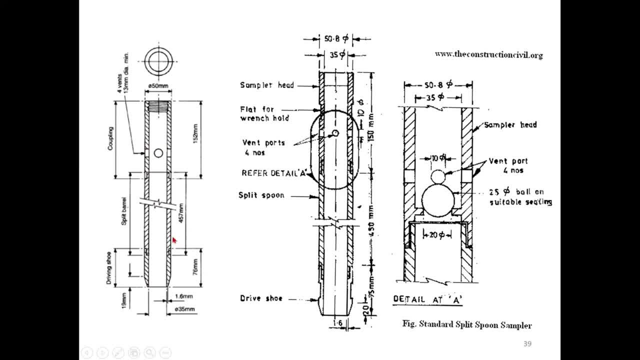 So this can be thick walled or thin walled. Okay. So, as I mentioned this thread, it will be connected to the tip of the drill road and it will be driven down at the bottom of the borehole. Okay, So you will use a churn bit or a cutting edge to make a borehole. 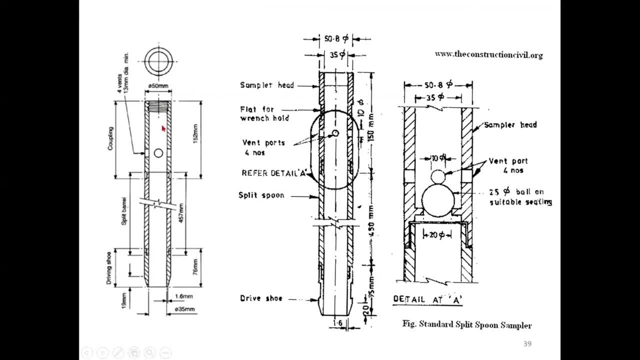 Then you will remove the churn bit, or cutting edge, and you will fix this splice spoon sampler. Once this is fixed, then you will drive this into the soil. Okay, This is driven into the soil. So once you retrieve the sample, it will be sealed. 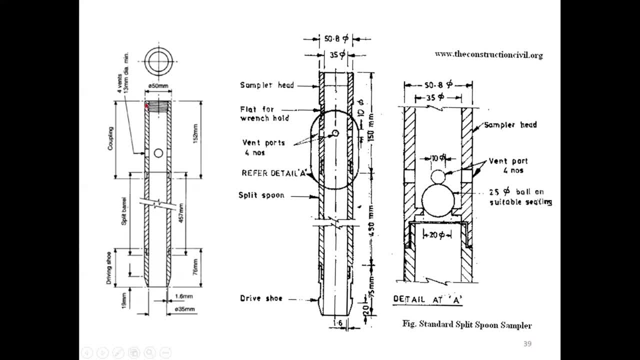 Both the top and bottom will be sealed with grease or molten wax- paraffin wax- after extracting So thick walled splice spoon samplers if it is thick walled. thick walled samplers are used for obtaining disturbed samples, but representative by you know the walls will be pretty thick. 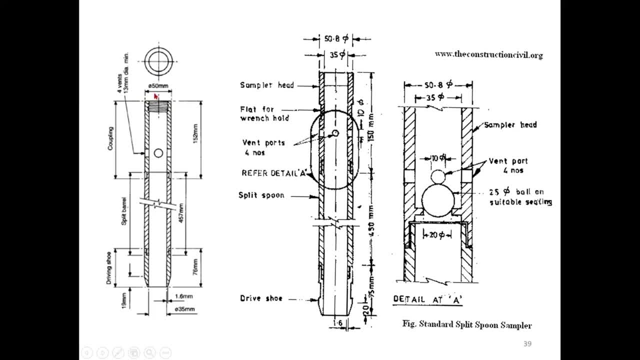 And this will be driven into the soil by repeated blows of a falling bait. Okay, You will keep this on the at the bottom of the borehole and, using the drill rod, some, you know, you will apply the impact using dropping weights. 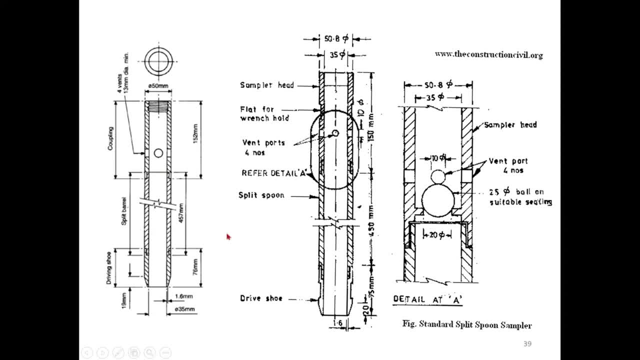 And this is driven into the ground and you, the samples that you obtain will be disturbed samples, but it will be representative samples. right, You will obtain representative disturbed samples And you can also use thin walled samplers. So thin walled samples are used of anti-corrosion materials like brass, aluminum, etc. which is having suitable strength so that it does not break or bend during the insertion and extraction. 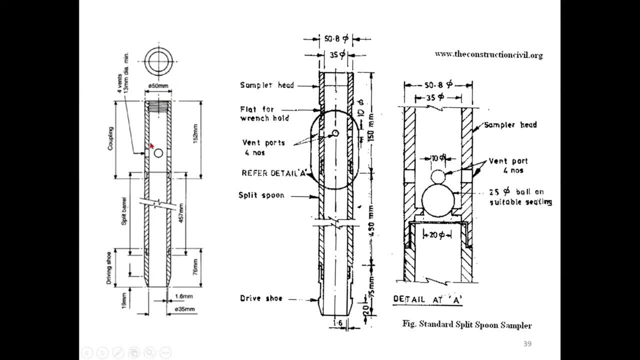 So this is pushed in with a constant, Okay, Rapid motion, without impact or twisting. If it is thin walled, okay, Because if you are using a thin walled, our objective is to obtain an undisturbed sample. So if it is a thin walled sampler, you will not, you know, use a dropping weight to drive this into the ground. 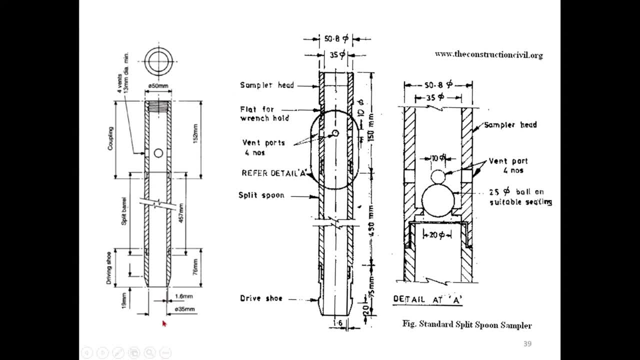 You will just push it into the ground And so that the sample smoothly enters inside this and then this is retrieved. Okay, So you have thick walled and you have thin walled. you will use a dropping weight to uh as an impact to hit and drive this into the ground. 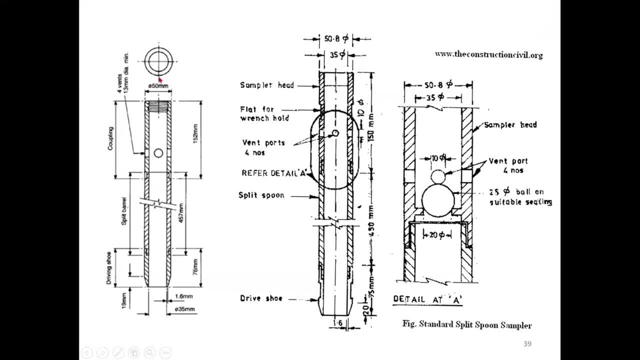 Okay, So you can drive this into the soil, or you can uh stationarily, you can uh using a piston. you can drive this into the soil as well, All right, So thick walled and thin walled, uh, so uh, you will uh use this. you will remove your churn bit and uh connect this and collect the samples at a depth of every uh 0.5 to 2 meters or whenever you find a change in the soil strata. 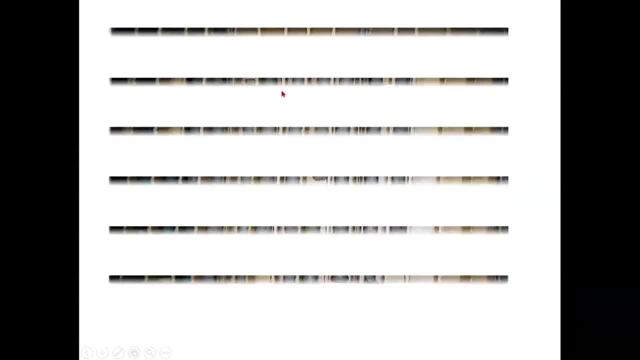 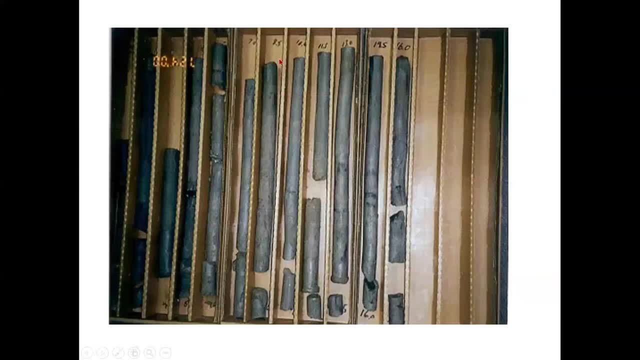 Okay, Whenever you detect a change in soil strata, you will collect a sample. So, from different depths you will collect the samples like this: and, as I have shown earlier, for different depths, you will collect all these samples. uh, at different, at change of strata, or every two meters, you will collect samples. 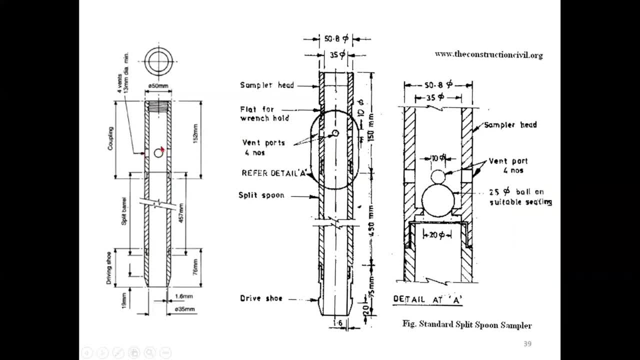 All right, Then another very important uh part is this: air vents. Okay, You can see air and water vents. you have these four vents, so that it is uh, you know, imagine uh, you are driving a- uh water bottle upside down into a bucket of water. 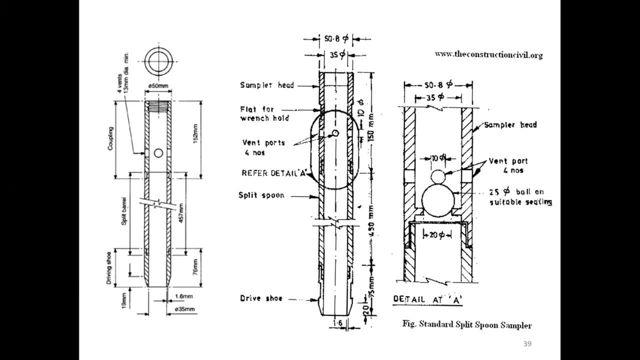 Okay, You cannot drive it down, Isn't it? So now can you drive a water bottle, open water bottle upside down directly into the bucket of water? No, Right, Why? Because there will be pressure formed inside the water, right? 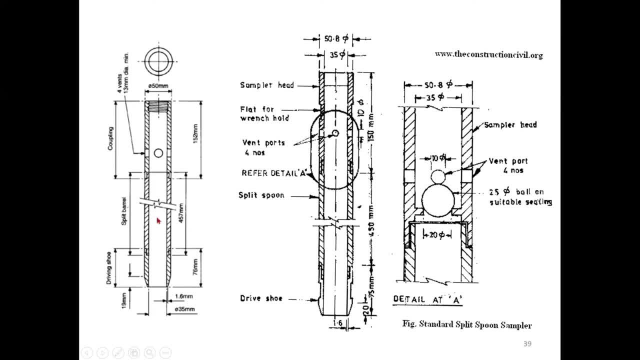 Similar concept here. So if you're driving it into the soil, the soil has to displace this air and it has to take this place right. So you have these vents here, so that when you're driving this into the ground, the air is removed to you through these vents and the soil sample easily, without any. 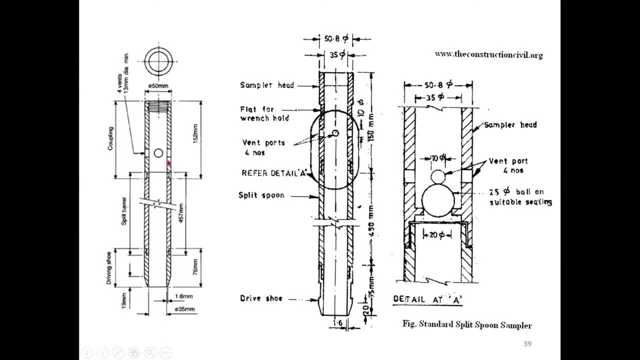 Distraction, Disturbance, it will slide in. Okay. Similar case for excess water in the soil as well. excess water in or ground water in the soil as well, Okay. So when you are driving this into the soil, the water will be- uh, you know- gushed out through these vents and the soil sample can easily be accommodated inside. 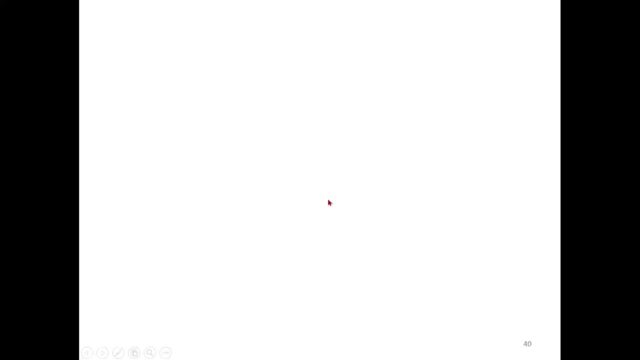 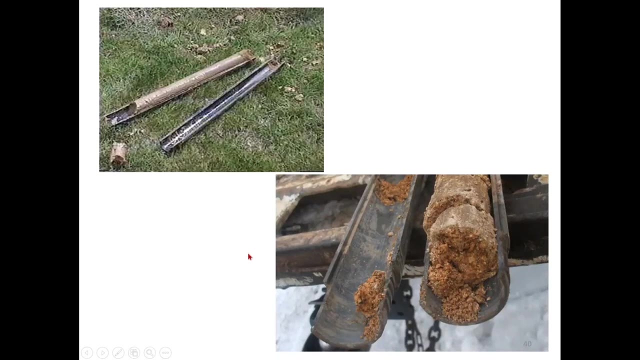 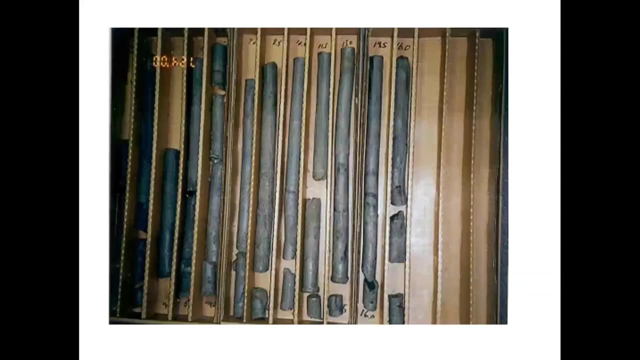 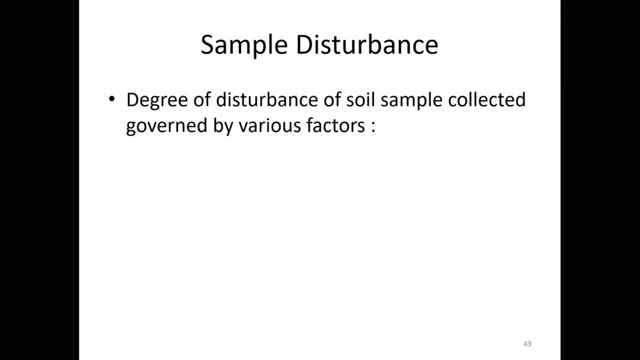 So that is why we have this air or water vents. Okay, So this is my splice Swim sampler sample collected inside. You can see, Right, These are samples collected at different depths, different samples collected. So the sample that you are collecting, you should make sure that the disturbance is minimal. 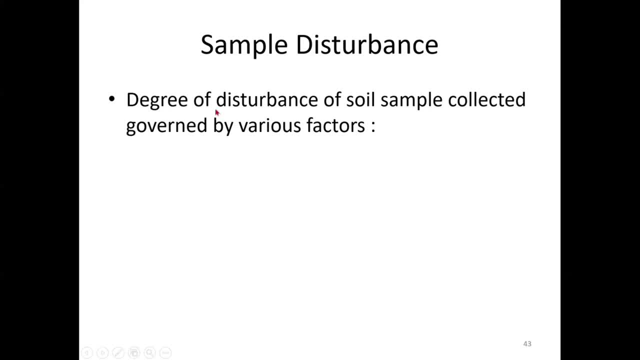 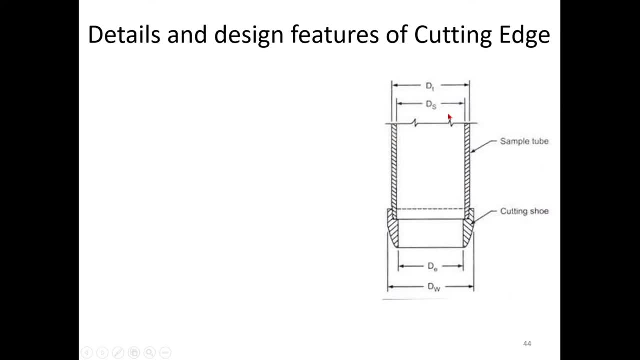 So this sample disturbance is governed by various factors. So if you look at the, if you look at your split spoon sampler, there are a few dimensions that you are you should be available about, I mean you should be aware about. So this you can see. here you have DE, that is, this inner diameter of the cutting edge. 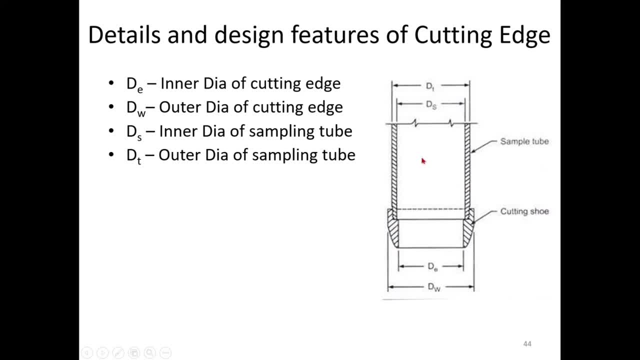 DW. outer diameter of the cutting edge, then inner diameter of the sampling tube DS and outer diameter of the sampling tube DT. Details and design features of the cutting edge. these are the sizes notations for a sampler. So these are the features. 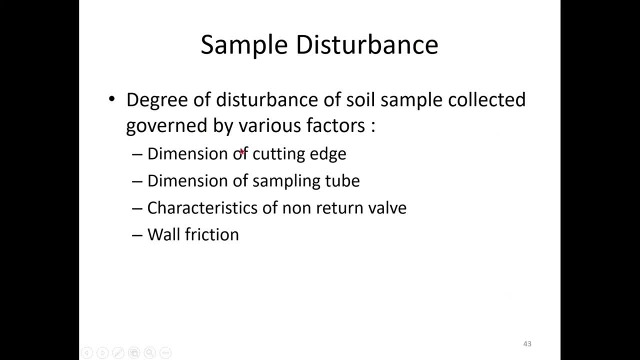 So before that, the sample disturbance, it is actually governed by different factors. One is dimension of the cutting edge, as I just showed you now, dimensions of the sampling tube, dimensions of the cutting edge and sampling tube I just showed you now. then characteristics: 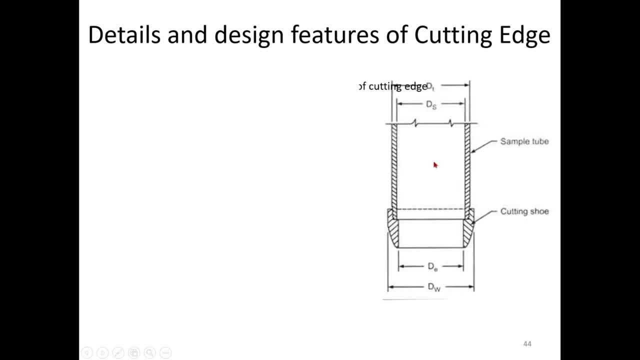 of the non-return valve and valve friction. So characteristics of the valve here. I showed you the air valve earlier, so characteristics of that valve and valve friction. how much friction is developed while you are inserting this into the soil? All right, So here you can see that, the sampler, cutting edge and sampler dimensions DS and DT and. 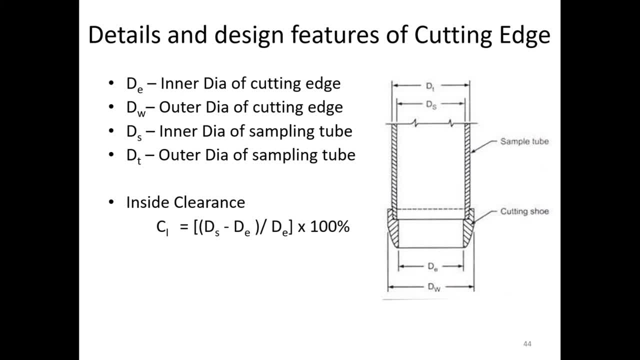 DE and DW. So some parameters, design features or parameters for the sampling tube. you can see there are four different parameters. One is an inside clearance, another one is outside clearance. So inside clearance is nothing but DS minus DE. So DS is inner diameter of the sampling tube. 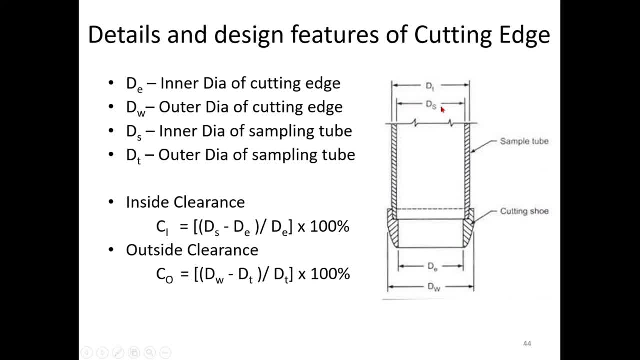 DE is inner diameter of the cutting edge, Sampling tube diameter minus cutting edge diameter by cutting edge diameter into 100% as a percentage. All right, So that is my inside clearance. Then outside clearance, DW minus DT, that is outer diameter of the cutting edge, and 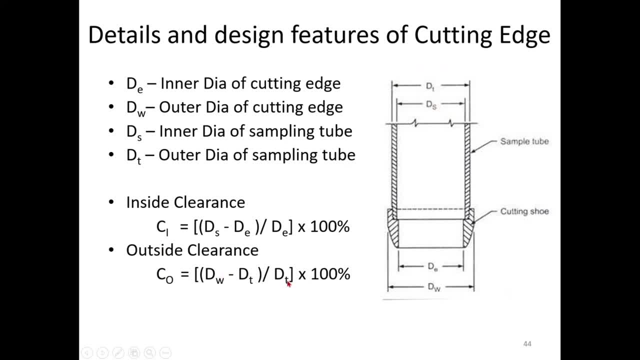 outer diameter of the sampling tube. So DW minus DT by DT, represented as a ratio of the outer diameter of the sampling tube, DW minus DT by DT as a percentage, Then I have area ratio. Okay, Area ratio, that is DW square minus DE, square by DE, square into 100.. 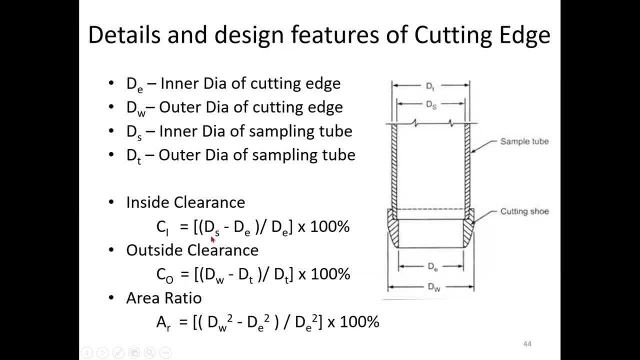 So these three parameters you should be aware of. Okay, What is important? I will tell you. So: inside clearance: DS minus DE by DE. Outside clearance: DW minus DT by DT. and area ratio: DW square minus DE square by DE square. 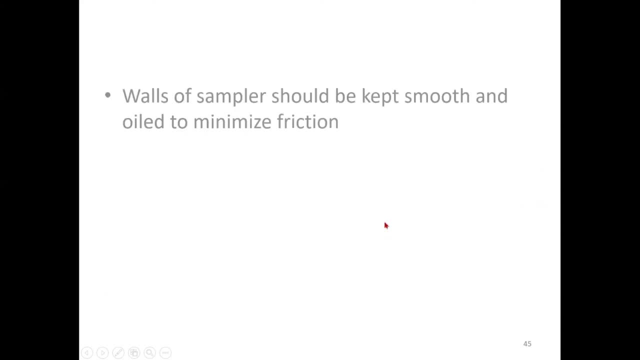 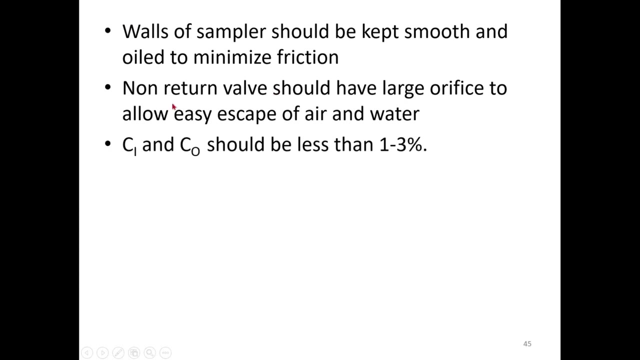 Okay, These are the few parameters of the cutting edge you should be aware of. And Another thing is that the walls of the sampler should be kept smooth and oiled to minimize friction, All right. And non-return valve should have a large orifice to allow easy escape of air and water. 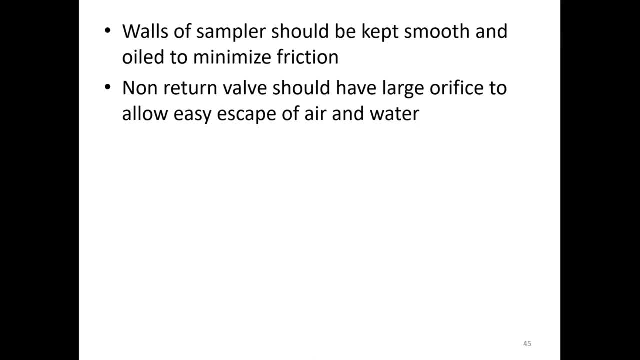 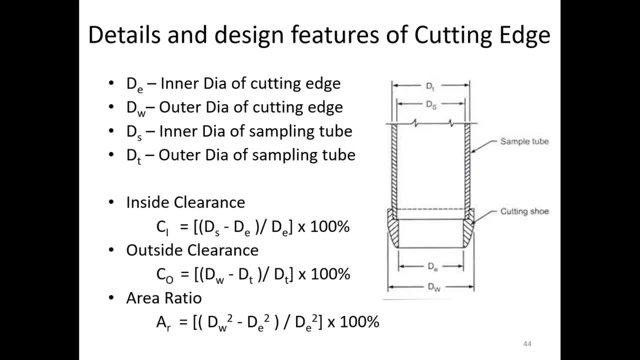 So what were the parameters that you should be concerned about to reduce the sample disturbance? So one was the dimension of the cutting edge. all right, these dimensions, dimensions of the cutting edge, dimensions of the sampling tube, then characteristics of the non-return. 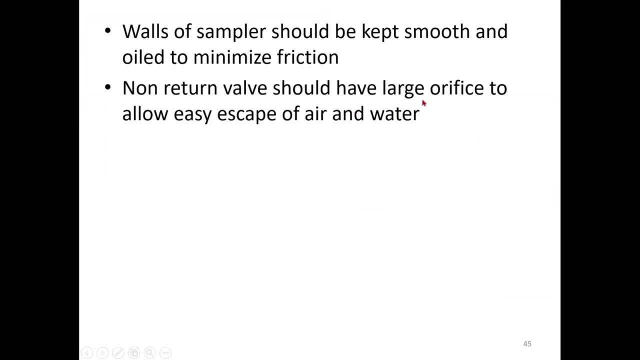 valve I mentioned here. The non-return valve should have a large orifice so that water and air is easily escaped, And the walls? another one was wall friction, So walls of the sampler should be kept smooth and oiled to minimize the friction. 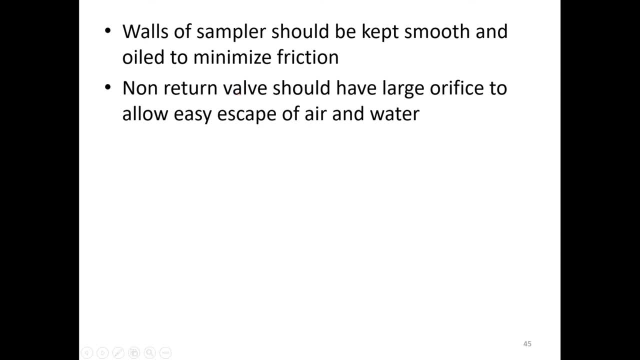 So if there is more friction the sample is going to break and get disturbed again. Right, So it should be greased well. greased well so that the friction developed is minimal. All right, So the CI and CO, it should be less than one to three percentage. 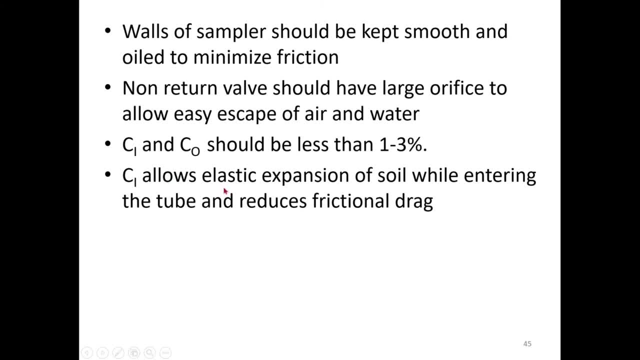 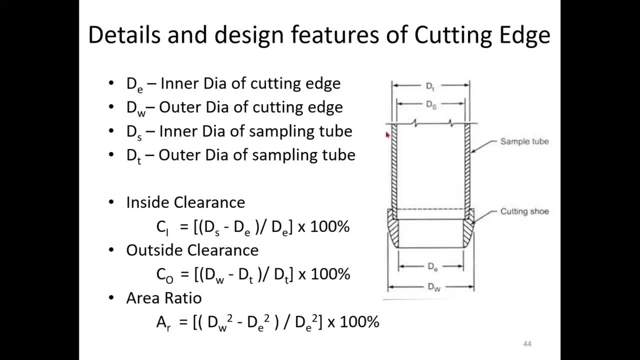 And why? Because The CI or the inside clearance. it allows the elastic expansion of soil while entering the tube and reduces frictional drag, As you can see here. the inside clearance, it is a difference between inner diameter of the sampling tube and inner diameter of the cutting edge. 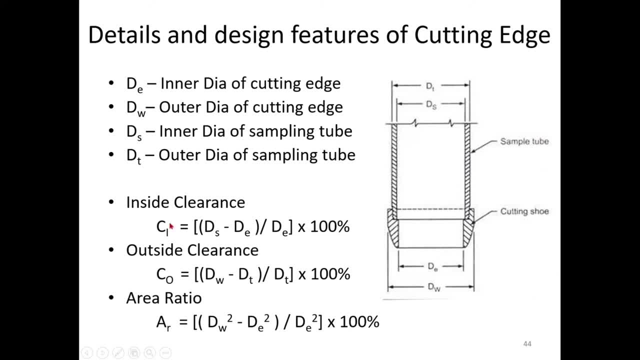 All right. So this ratio is represented as inside clearance, So that should be one to three percentage only. So why you need some inside clearance is because, as you can see here, As the sample enters this tube, you should provide some space for elastic expansion. 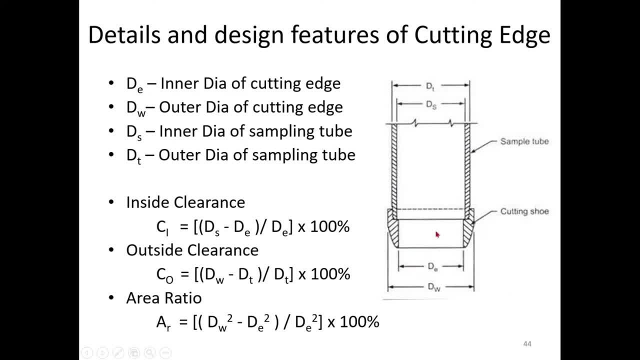 of the soil Right. So once the sample enters this cutting edge and enters this tube, there should be enough clearance for the sample to expand. All right, So that the frictional drag inside will be minimal. All right, So that provision should be provided and that is given by the inside clearance. 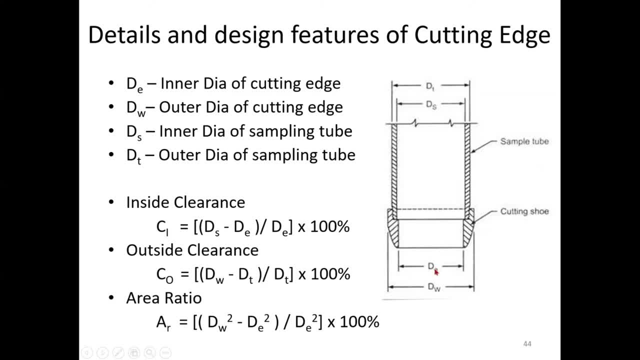 Okay, So you can see it is ds minus de. So it will provide some clearance inside the inside clearance for the sample to allow it for some elastic expansion and reduce the frictional drag while entering into the tube. All right, Next one is outside clearance: dw minus dt. 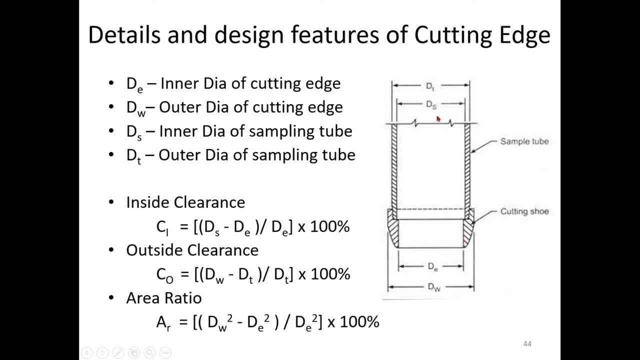 So that allows easy withdrawal of the sample from the ground. So once you insert, this sample enters, and once you retrieve this, it will be easy for removing the sample. That is why you need the outside clearance. Okay, Then next one is the most important parameter: the area ratio ar. 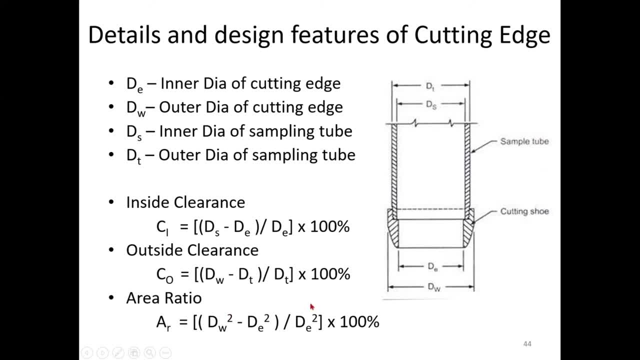 So it represents the ratio of the displaced volume of soil. It represents the displaced volume of the soil to that of the sample collected. area ratio: It represents the ratio of displaced volume of soil to that of the sample that is collected inside. How much volume of soil is displaced while you insert this tube? 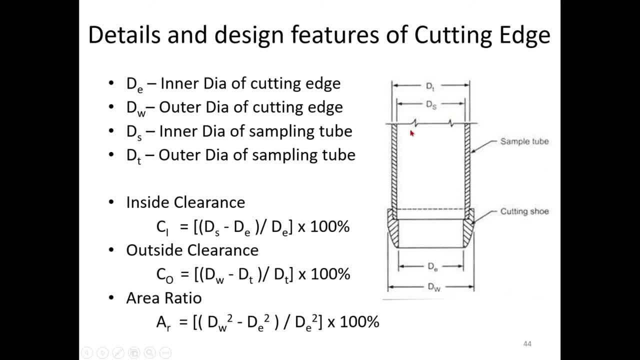 Compared to the volume of the sample that is collected inside this, All right. So if the area ratio is less than 10 percentage, then we can say that the sample disturbance is less Okay, And if it is a thick walled sampler, then the area ratio may be as high as 30%. 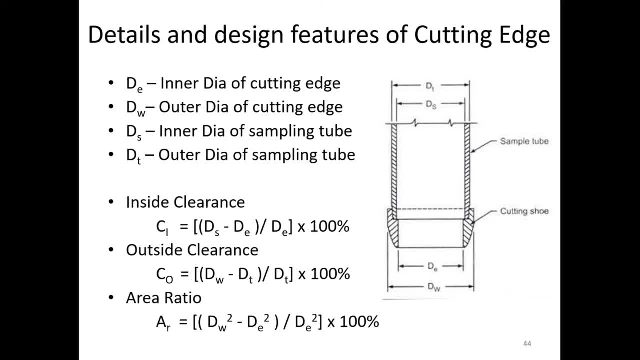 I told you earlier, If it is a thick walled sampler, the sample disturbance will be high right. So if the area ratio is about 30% For thick walled samples and for thin walled samples samplers, it can be as low as 6% to. 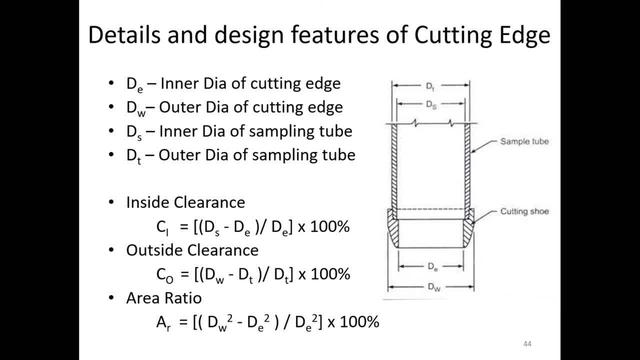 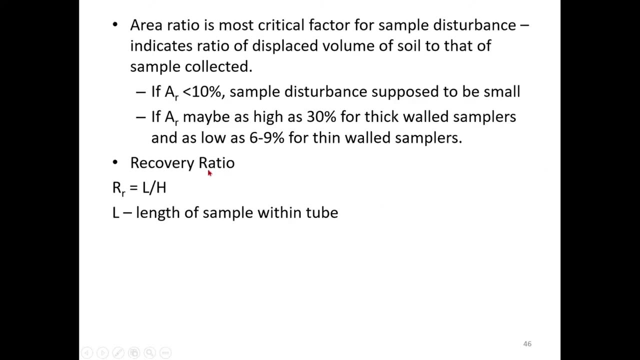 9% also. So an advisable area ratio for collecting an undisturbed sample is that the area ratio should be less than 10%. Okay, So that is the importance of CI, CO and AR. Okay. Next parameter is recovery ratio. 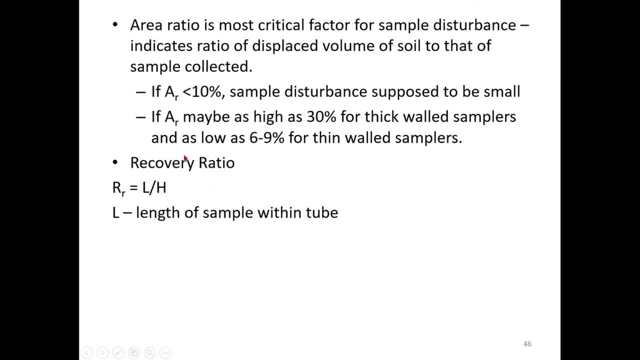 This is generally used for rock core samples. So recovery ratio RR is equal to L by H, where L is the length of sample within the tube and H is the depth of penetration of the sampling tube. So H is depth of penetration. If your tube is, let me say, 0.5 meters, you are inserting, you are penetrating the sampling. 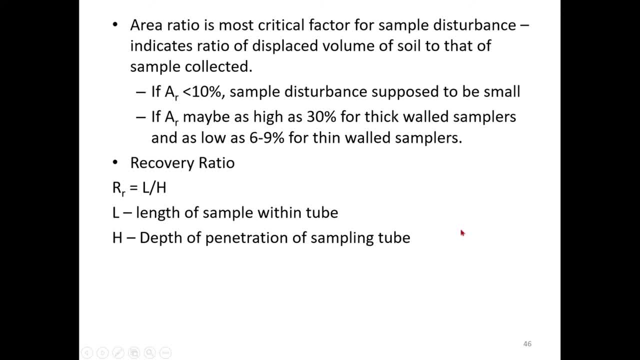 tube for 0.5 meters, But the sample that is collected inside is only 0.4 meters. The rest of the sample has broken away, All right. So the length of sample within the tube is 0.4 meters and depth of penetration of the 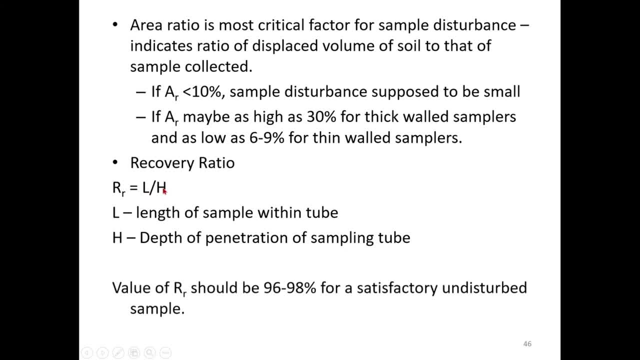 sampling tube is 0.5 meters. So what will be your recovery ratio? It will be 0.4 by 0.5.. Right, So similarly, for a satisfactory undisturbed sample, the value of RR should be 96 to 98%. 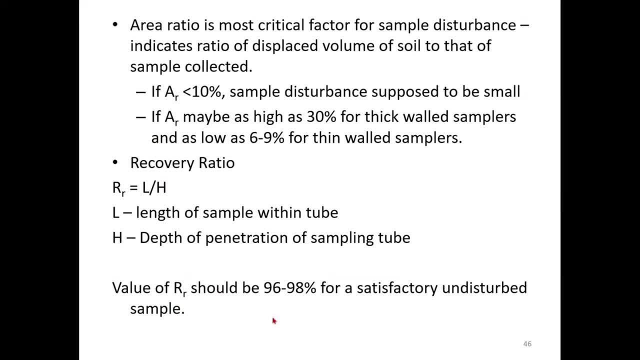 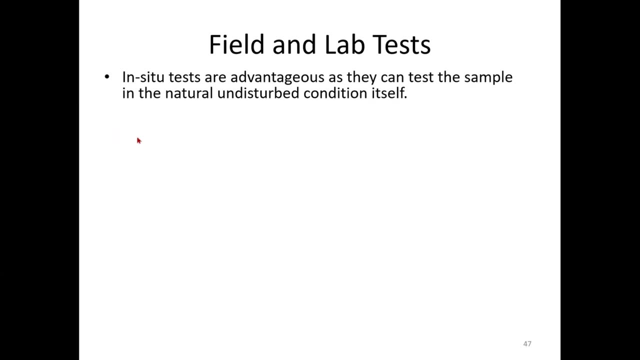 this L by H into 100 percentage. All right, So the value of recovery ratio should be 96 to 98% for a satisfactory undisturbed sample. So this is basically used for retrieving rock core samples. Okay, So next comes the field and lab test. 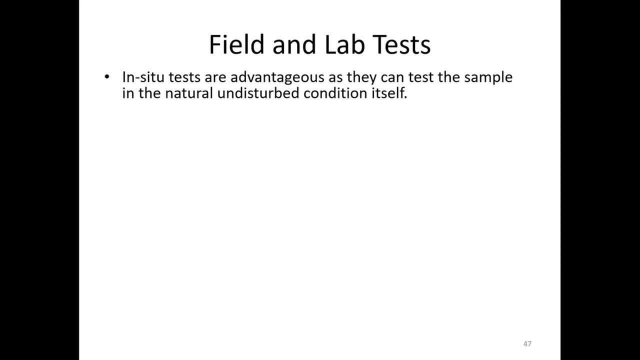 So we know that, however carefully you collect samples from the site, there are going to be some disturbance to the samples, isn't it? So you always try to test the samples at the field itself, in the field itself, so that the sample disturbance is minimal and you can test it in their in situ condition, with 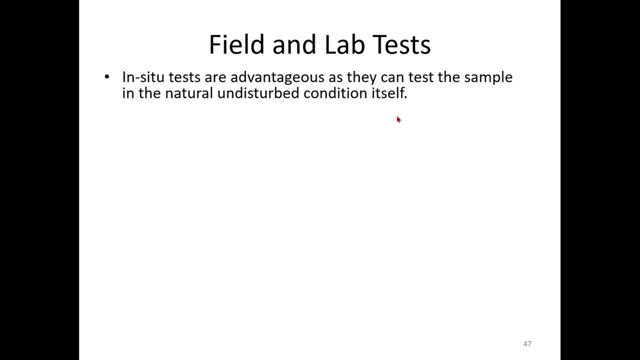 in situ parameters itself, right In its natural undisturbed condition itself, And also collecting undisturbed samples. it's very difficult to obtain samples from non-cohesive granular soils, isn't it? Non-cohesive granular soils? purely sandy soils? 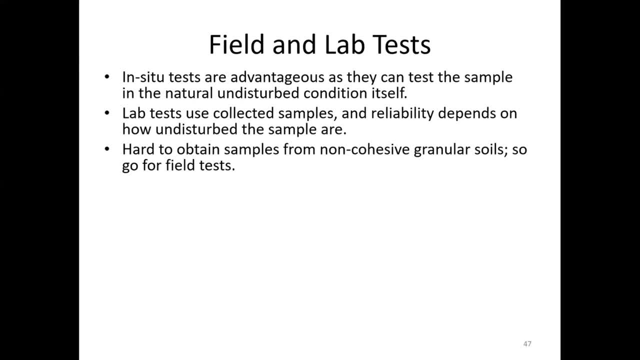 It's very difficult to collect a sandy soil sample inside a split spoon sampler, isn't it? You insert the sampler, the soil will be filled inside. You remove the sampler, the soil will simply drain out, isn't it? Yes or no? 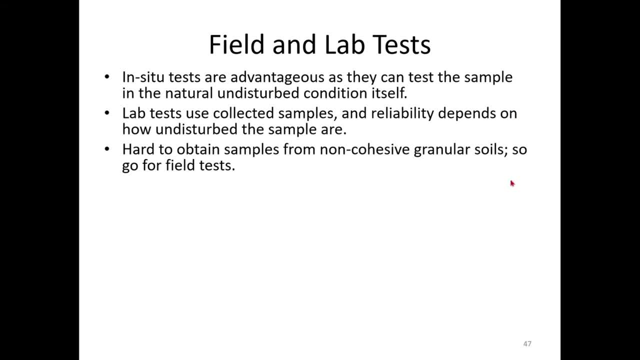 So it is very difficult to collect non-cohesive granular soil samples from the field or undisturbed samples from the field. So in such cases it's always advisable to go for field Field tests. but however cohesive soils, generally samples are collected because cohesive 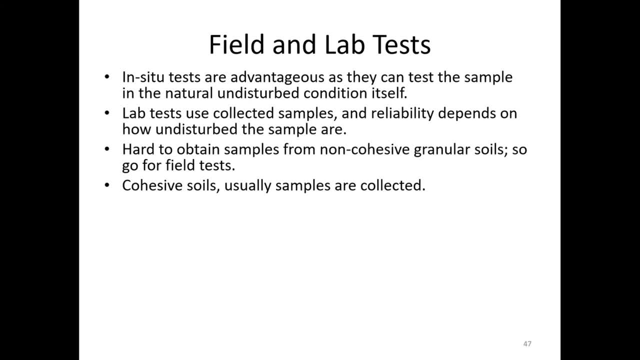 soils, clay soils. it's very easy to cut them into different shapes and you know you can use a split spoon sampler. You can get a block sample, chunk sample, anything you can get, because you can cut it into different shapes and sizes and they will stay intact when compared to that of a purely 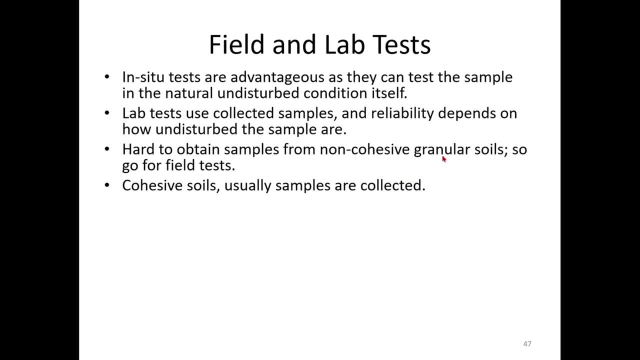 sandy soil, isn't it? So usually for non-cohesive granular soils you will go for field tests and in the case of cohesive soils, usually you will collect samples, So data from the field test. I told you we will do tests in the field itself. 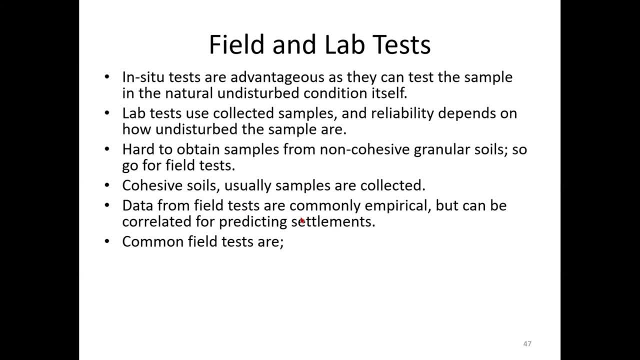 So those test results, using those test results, we have so many empirical relationships that can be correlated with the different soil properties or parameters like settlement or shear strength etc. Right, We have several empirical formulas developed by several researchers in the past. So maybe a penetration resistance in the field can be correlated to the shear strength of. 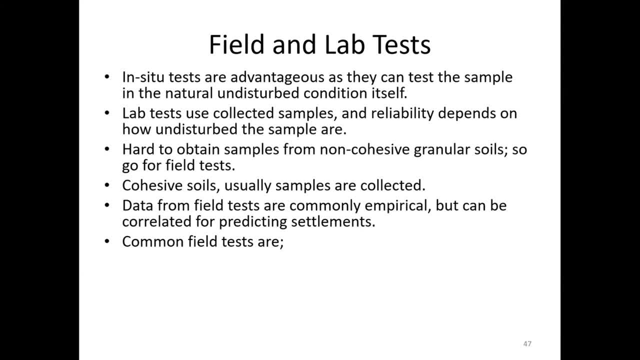 the soil. For example, vane shear test we saw, isn't it? Do you remember vane shear test? You measure the torque for driving the vane into the soil and that is related to the shear strength of the soil right. 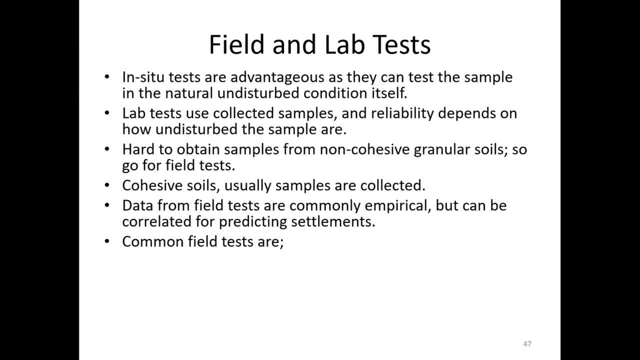 So there we saw an empirical relation. there we saw an equation connecting the same right. So there are different equations like this for different field tests which can be correlated to different soil parameters like shear strength, settlement etc. So there are several field tests available. 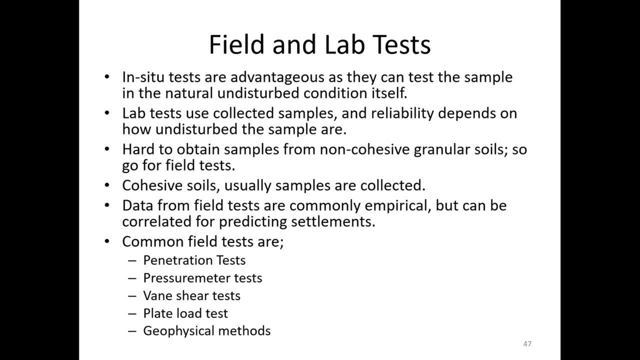 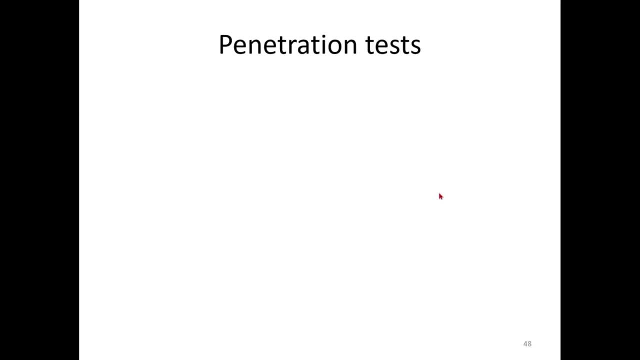 So a penetration test, Pressure meter test, vane shear test, plate load test and several geophysical methods are also there. So we will see all these. Okay, Many common penetration tests are that there are three common penetration tests, So there are three types of penetration test. 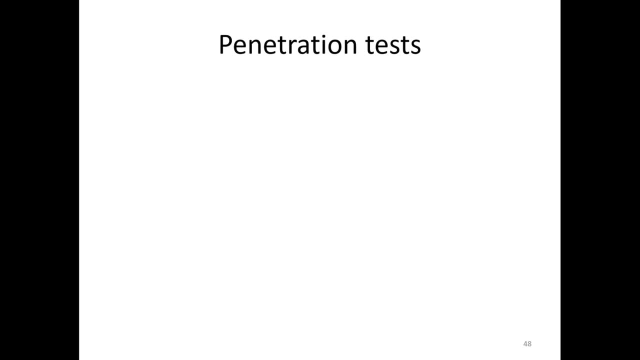 One is SPT, then DCPT and SCPT. SPT is standard penetration test, DCPT is dynamic cone penetration test and SCPT is standard static cone penetration test. So we have three different penetration tests. So the most commonly used one, very commonly used one, is my standard penetration test. 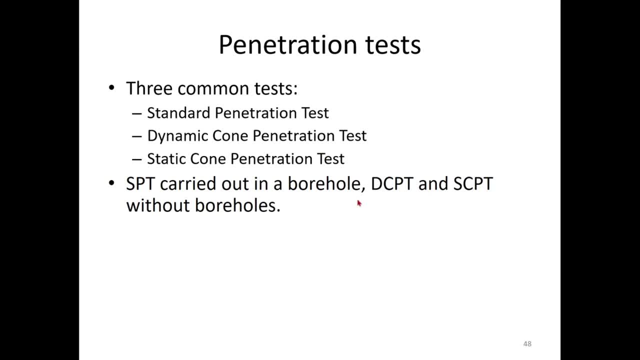 So standard penetration tests are carried out in borehole. DCPT and SCPT are used without boreholes. Okay, So what you basically do in penetration tests are: you will measure the resistance of the soil strata to penetration by a penetrometer and then, as I mentioned earlier, you have 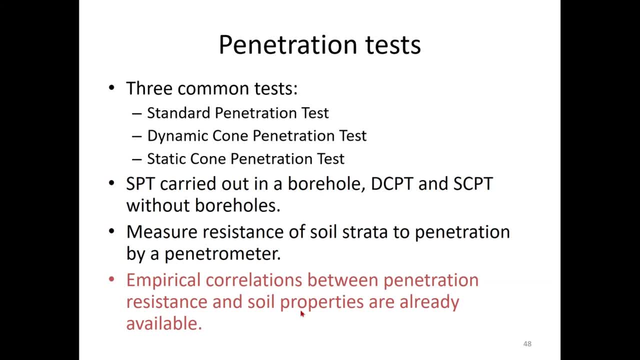 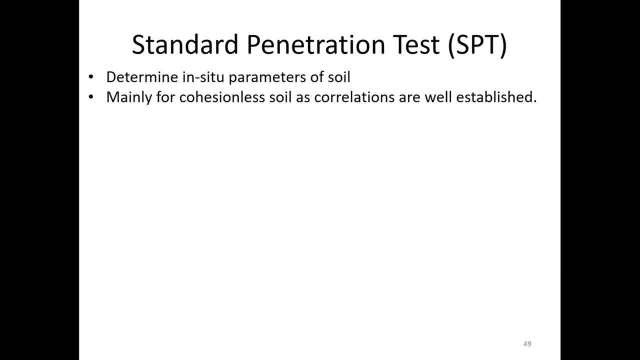 so many empirical correlations between this penetration resistance and the soil strength, So you will correlate those with those empirical relations and you can deduct some soil parameters. Okay, This is what is done in standard penetration test, DCPT and SCPT. So first one is SPT, or standard penetration test. 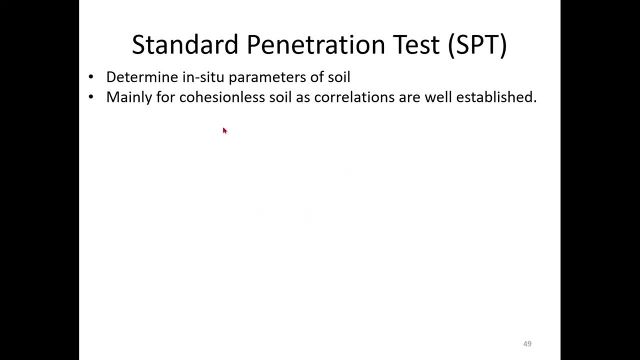 So it is used to determine the in situ parameters of the soil, basically used for cohesionless soils, as the correlations are very well established. The empirical: there are many empirical relationships which are very widely accepted by many geotechnical engineers. So usually standard penetration tests are adopted in cohesionless soils. 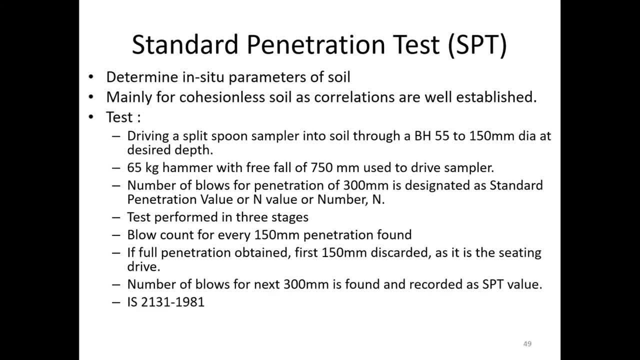 So how the test is done. It's very simple. I'll show you. So note this: IS 2131, 1981 mentions the specifications for standard penetration test. IS 2131, last revised in 1981.. Okay, All right. 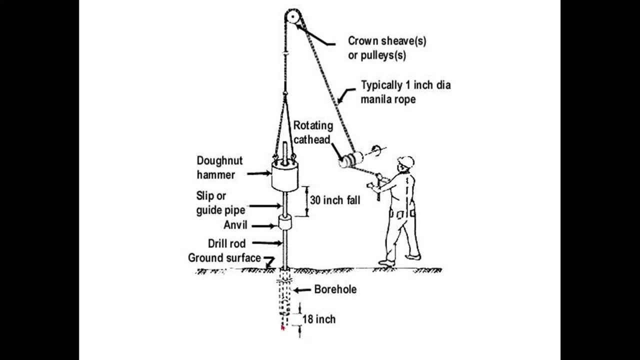 So let's see this. Yeah, So you can see. here you have a borehole of 55 mm to 150 mm. You have different size The borehole. So basically a borehole ranges from 55 to 150 mm. So let's say we have this borehole then at the bottom of the drill road, 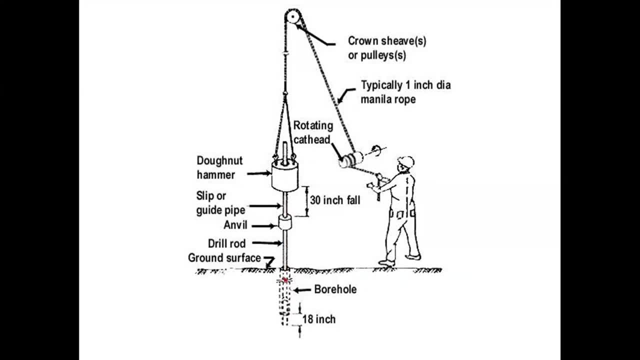 This is my drill road. at the bottom of the drill road, What do I have? I have a split spoon sampler. Okay, I have a split spoon sampler at the bottom, Then I have an. I have a drill road, then I have an anvil, then I have a guide pipe, then I have a. 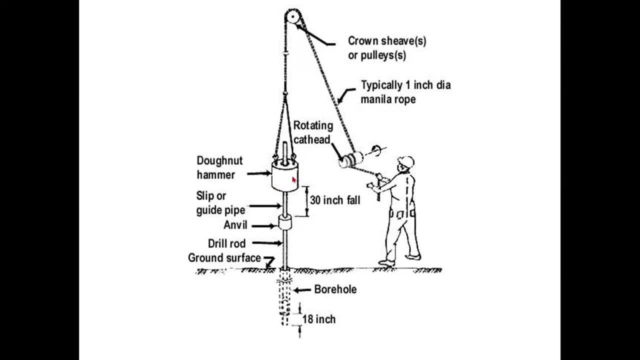 weight hammer. All right, then I have a pulley and winch system. then I will pull this. So this is raised, I drop this, so this free falls to a height of 750 mm. This hammer is 65 kg in weight. This is 65 kg and this free fall height is 750 mm, 75 centimeters. 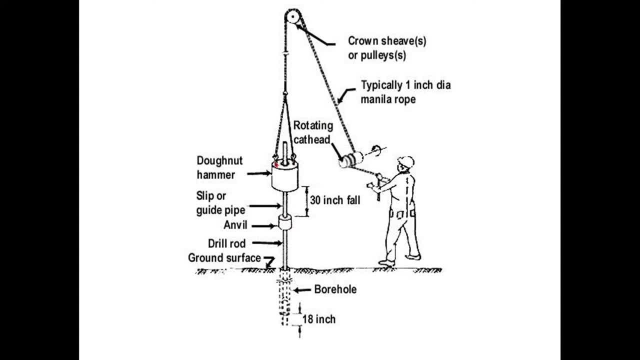 So I will raise this to a height of 750 mm. I will drop this. This is a 65 kg hammer, So it will hit this anvil and this split spoon sampler is driven into the ground with each impact. Okay, So what you are going to measure here is you will Mark 150 mm on the roads. 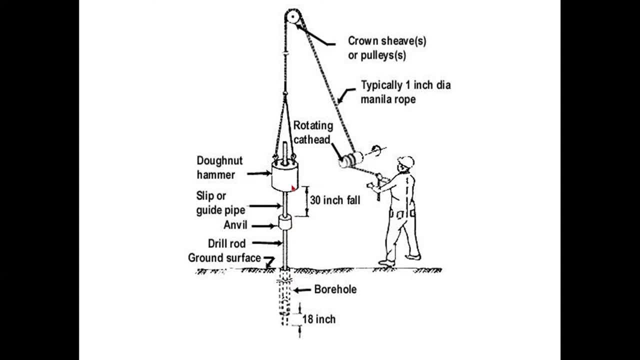 Right, you will hit it, And how many number of blows? using a 65 kg hammer and a free fall height of 750 mm? how many number of blows are required To drive the split spoon sampler to a depth of 150 mm or 15 centimeter? 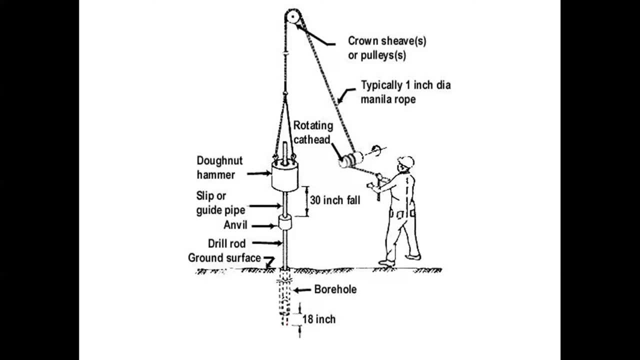 This is what is measured in this test. Okay, the number of blows required by a split spoon sampler to be driven into the soil for 150 mm using a hammer of 65 kg falling through a free fall height of 750 mm. that number of blows is represented. 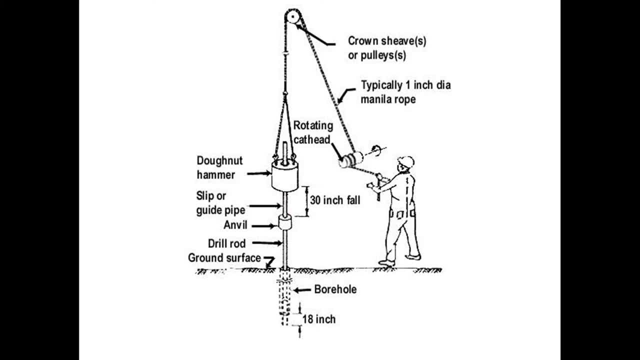 as this N value or SPT n value, not just for 150 mm. You will do that test for three times: 150, 150, 150, 450 mm in total and if you get 450 mm penetration- listen very carefully- if you get 450 mm penetration, you will discard the first 150 mm, as you will. 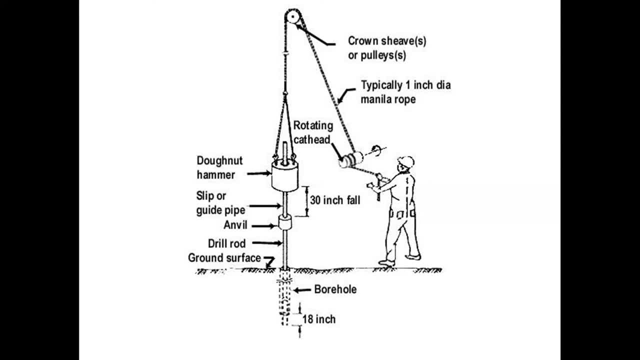 consider that as the seating drive, the rest 150 plus 150, 300. mm penetration. What are the? what is the number of blows required for that 300 mm? that is designated as the n value for that particular soil at that particular depth? Okay, suppose I have made a borehole. 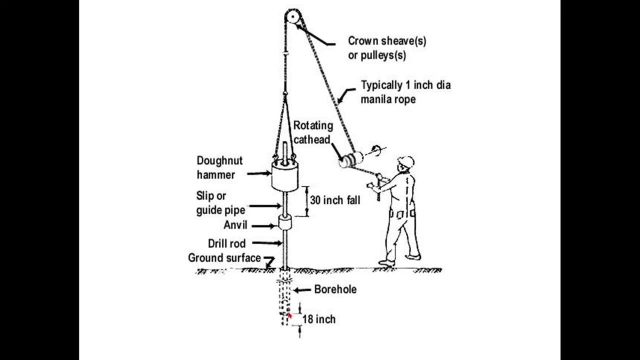 Let me say borehole is 1 meter at the bottom of the borehole. I'll make this borehole at the bottom of the borehole. What will I do? How will I make this borehole? I will at the end of the drill bit. 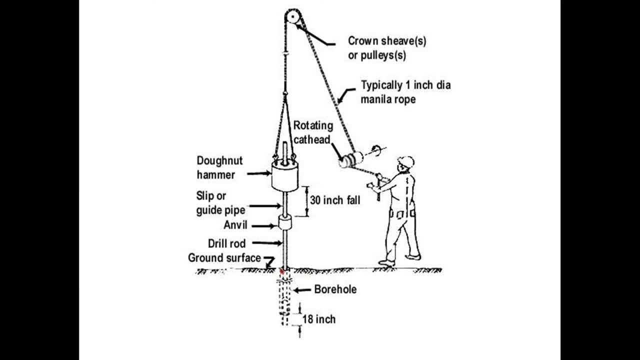 I will have a churn drill or a cutting edge, So I will Use any of the method: wash boring, percussion drilling, rotary drilling, auger boring- any method I will use and I will make a borehole. Let me say this borehole is 1 meter deep now. 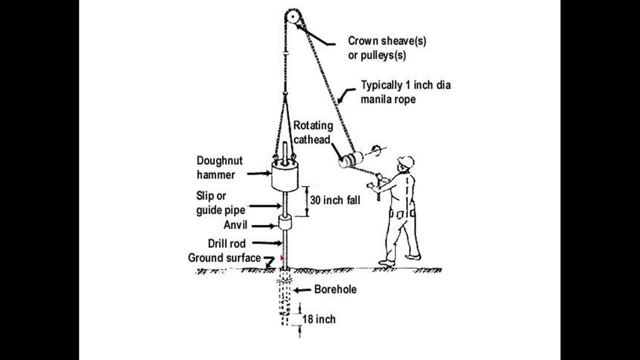 So what will happen now? I will remove this. at the end of this drill road I will connect my split spoon sampler. I showed you to has threats at the end edge, So I will connect that split spoon sampler. I will keep that split spoon sampler on the surface of the borehole. 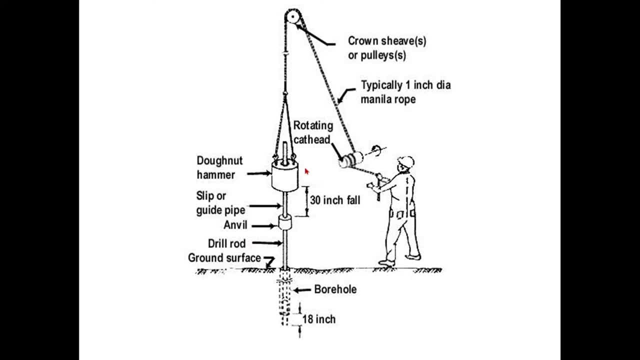 Then I will raise this and drop it and I will count. Okay, I will count. Okay, I will raise and drop it, I will count it. and for the first 150 mm penetration, How many number of blows? So let us say n is equal to 10.. 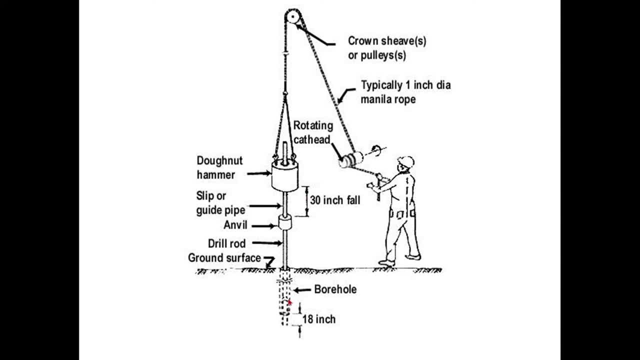 Okay, took 10 blows to drive it for 150 mm. Then I will keep on going: another 12 and another 12 number of blows for the next 150 mm. Okay, next I will again. I will continue again: another 10 blows for the next 150 mm. 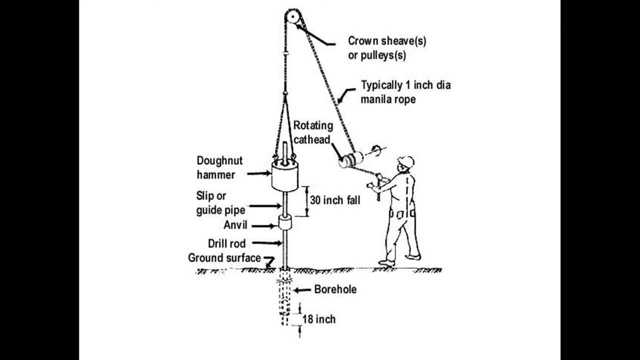 So I reached 450 mm. So the first 10 I will discard. So the second number of blows for the second 150 mm and the third 150 mm, It was 12 and 10.. So my n value at 1 meter depth is how much? 22.. 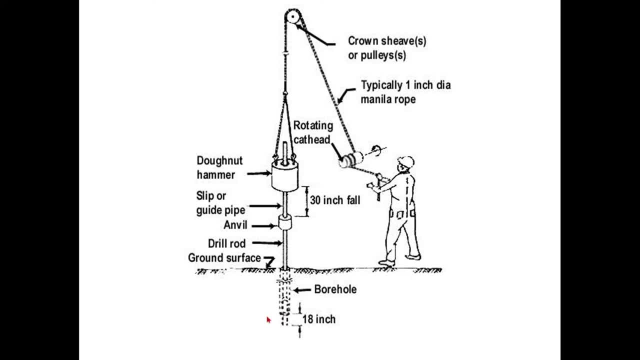 So that is my SPT n value at 1 meter depth of soil. All right, suppose. suppose I didn't reach 450 mm penetration, Suppose I had a hard rock here itself. Okay, maybe at 1.3 meters I had hard rock. 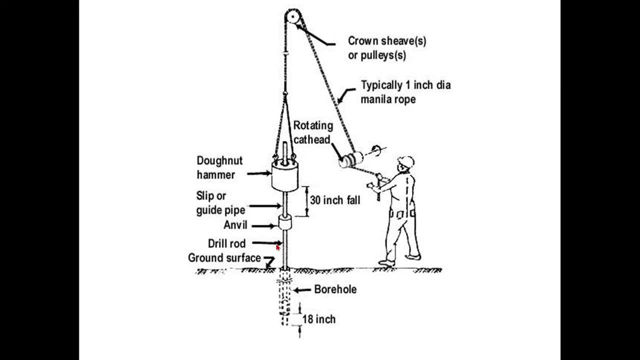 Okay, I am driving this. the first 150 mm, It went 10 number of blows. the first 150 mm, Then the second 150 mm. It took 12 blows and the third 150 mm was not reached. How many ever number of blows I gave, it couldn't penetrate more than 12 mm. 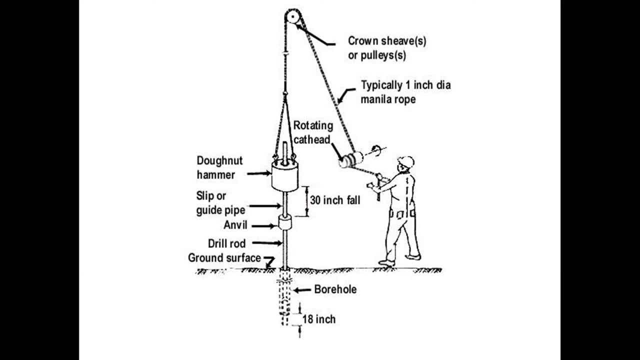 Let us say 12 centimeters, Let us see All right. So what I will do is at that depth, I will say that at that depth I have reached the refusal and the soil above that. The n value is 10 plus 12.. 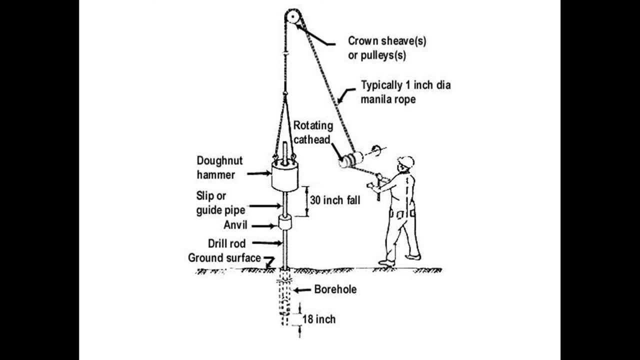 The initial 10 plus the next 12.. That is my n value at that particular depth, and below that I can say that I encountered refusal because for a n value greater than 50 for 150 mm drive or n value greater than 100 for 300 mm drive, if it is more than 50 for 150 mm or more than 100 for 300 mm penetration. 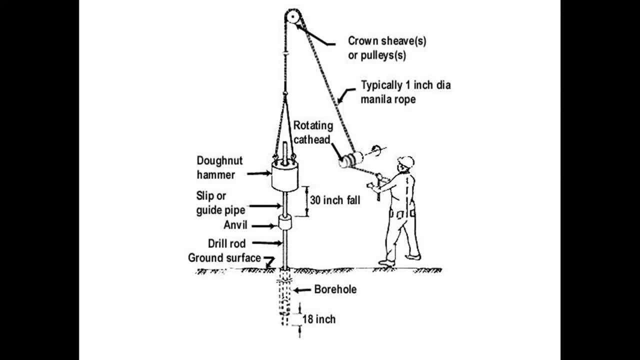 You will say that the you have Reached refusal level or hard rock strata. Maybe right, So that level is called as refusal. Okay, either you should go for more than 50 blows for 150 mm, or more than 100 blows for 300 mm, or no advancement. 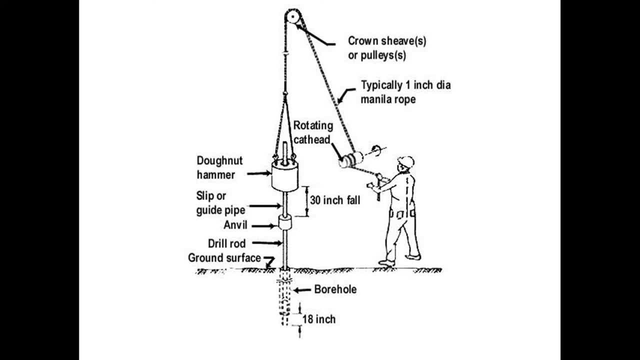 Also, you might not be a, might not even be able to drive 150 mm, So that that's called as no advancement. Okay, you cannot drive the sampler any further. So in all these three conditions, That is, n is greater than 50 for 150 mm, in is greater than 100 for 300 mm, or no advancement in these three conditions, 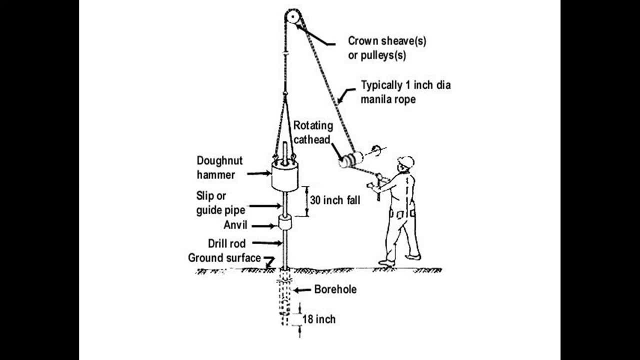 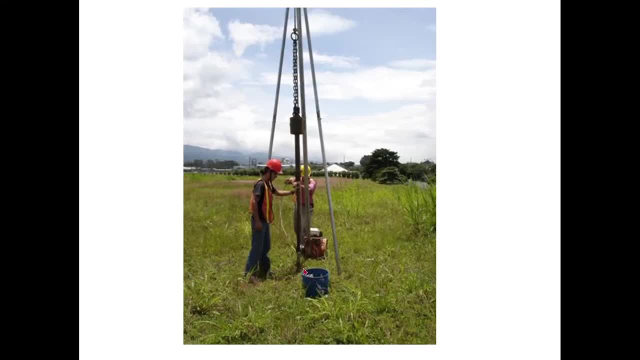 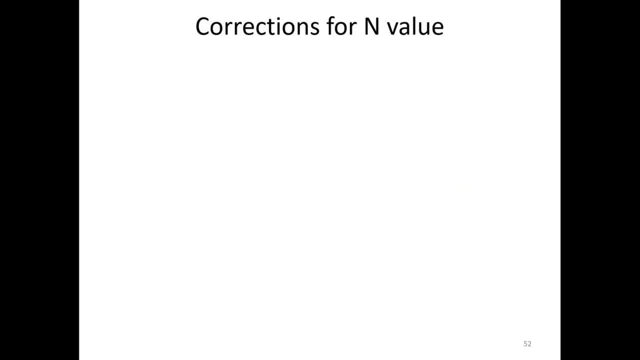 You will say that you have reached the refusal level. All right, Hope it is clear. All right, So this is a testing and value SPD test. So there need to be some corrections done for n value. All right, So there are two corrections for the n value. 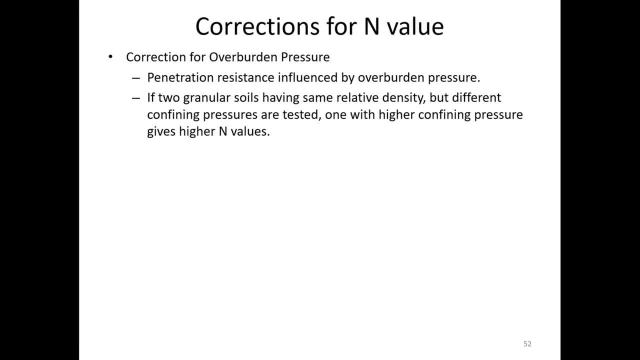 One is an overburden Pressure correction and the other one is a dilatancy correction. So the penetration resistance is actually influenced by overburden pressure. So as the self weight of the soil increases, the self weight of the soil increases with depth, isn't it? 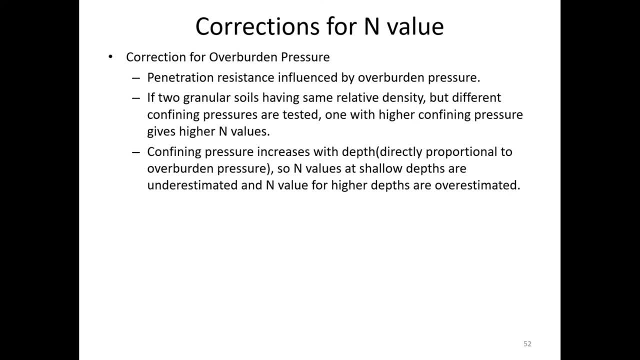 Right, because the overburden pressure at, let's say, our depth of H meters is gamma into H, isn't it? gamma is the density of the soil. So gamma into H, correct for 2 meters. It is gamma into 2 for 4 meters. 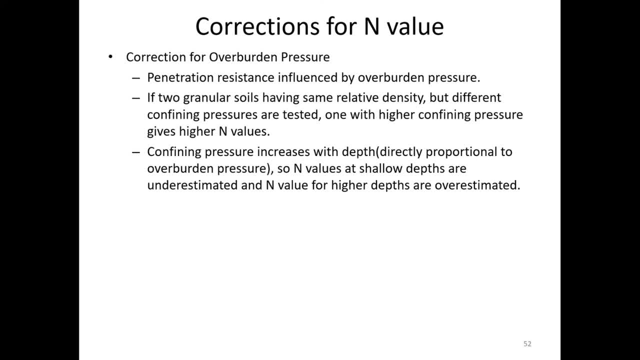 It's gamma, So overburden pressure keeps on increasing with depth, isn't it So this overburden pressure has a effect on the n value. So as the overburden pressure increases, the resistance of the soil also increases. agree, Correct, confining pressure increases with depth, isn't it? 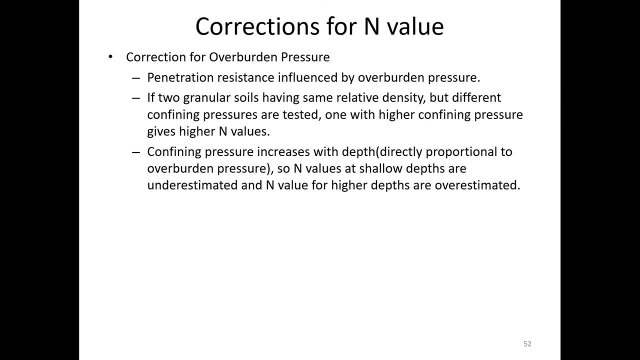 The pressure with which the soil at a deeper layers are confined. It is higher when compared to that at the shallow levels, isn't it Correct? The confining pressure at a deeper level is higher when compared to the confining pressure at a shallow depth. 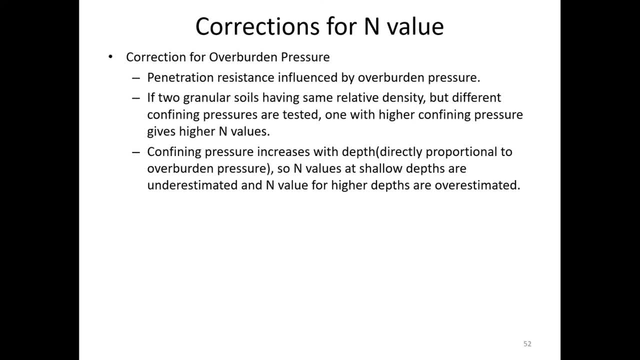 Do you agree with that? Yes, makes sense. So the overburden pressure is high at the base and high at higher depths, and it is low at the shallow depths. So this is going to influence your n value also, right? So if the confining pressure is higher, you might require more number of blows at a deeper depth. 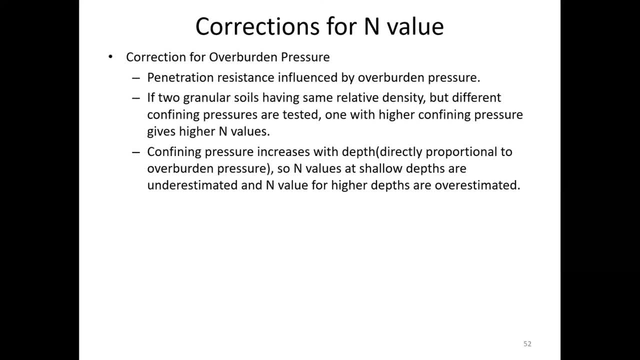 Correct and at shallow depth overburden pressure is very less, So the number of Blows required in the same soil, The number of blows required will be lesser. correct, So to correct this, using this concept, to correct this, you will go for a correction of overburden pressure. 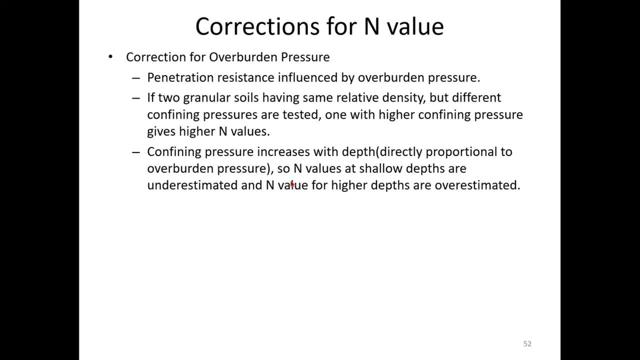 Okay. So as the confining pressure increases with depth, n values at shallow depths are underestimated and n values at the higher depths are overestimated, Correct. So to get a- you know- corrected n value, you have to apply the overburden pressure correction. 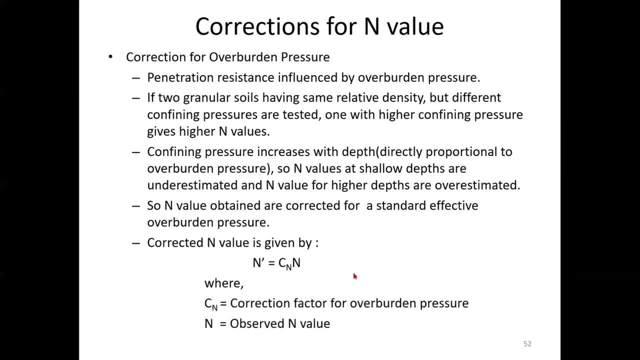 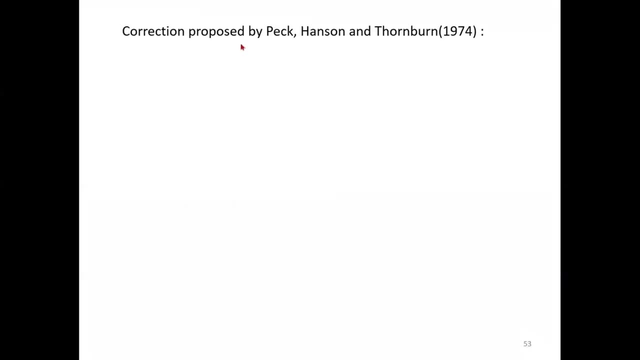 So that equation is given by n dash is equal to c N into n, where n dash is the n dash is the corrected, corrected spt n value. c N is my overburden correction factor and n is the recorded n value. Okay, and that c? n was. equation was given by Peck Hansen and Thornburn in 1974. 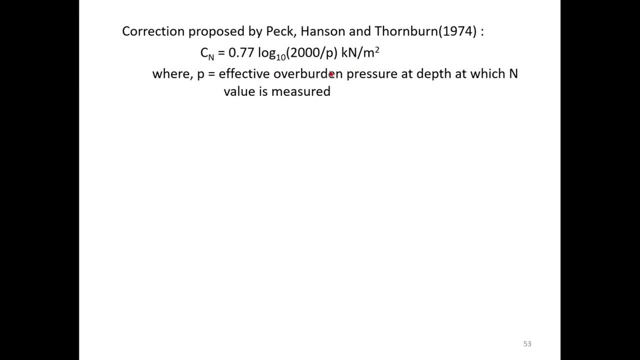 So the equation says: c: n is equal to 0.77 log 2000 by p, where p is the effective overburden pressure at depth at which n value is measured. How do you measure this Overburden pressure? very simple gamma into H, isn't it effective overburden pressure at depth at which n value is measured? 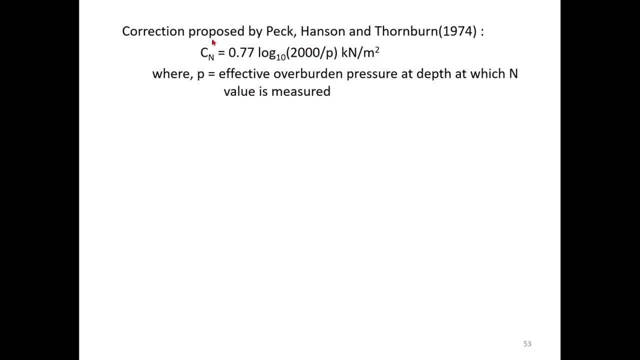 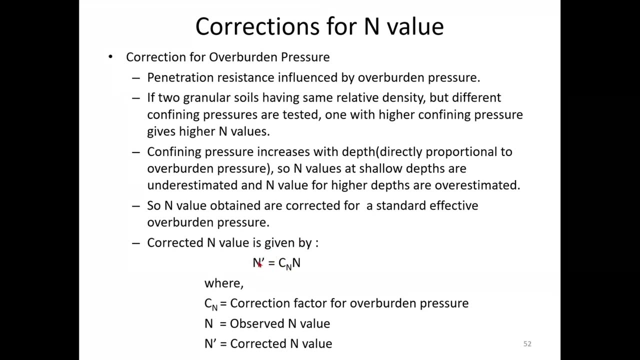 That is my p. substitute that p here. I will get my c n. so I get my c n. I substitute it here. I get my corrected n value: n value corrected for overburden pressure. All right, so that is my correction for overburden pressure. 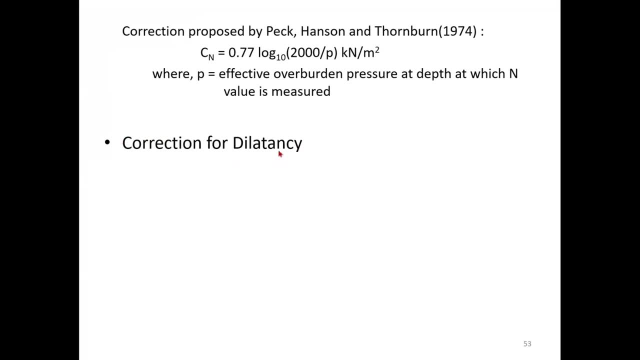 Next comes the correction for dilatancy. What do you mean by dilatancy? Something dilates means it expands, Right, We remember the behavior of dense sandy soil, the volume change behavior of sandy soil to strains. Initially the volume decreased very lightly. the volume decreased initially, then after that you saw increase in volume. 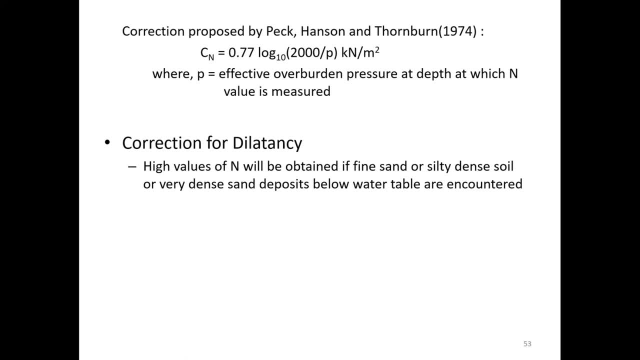 So you remember the volumetric change behavior, right. So, on application of some stresses, as the strain increases, What happens? initially there will be a small reduction in the volume. But after that, what happens? as the strain increases, what happens? the volume increase, right? The sample dilated correct. 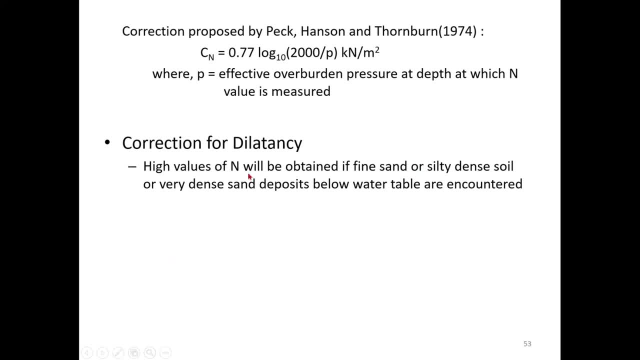 So same thing. if you are using this test you, if you are using SPT test in fine sand or silty, dense soil or very dense sand deposits below water table, What happens? the sample is going to dilate when you apply such strains, right? So there should be a correction for that dilatancy as well.